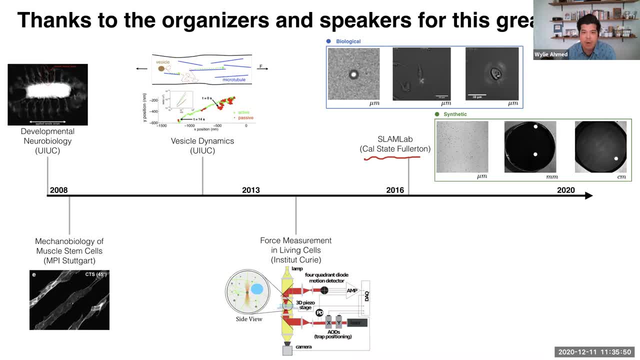 a primarily undergraduate institution. We have mostly undergraduates and a master's program, And I have a small army of students working on both biological systems as well as synthetic systems, And mainly the synthetic systems were motivated just so that we could cross different scales. And that brings us to today, where I'm going. 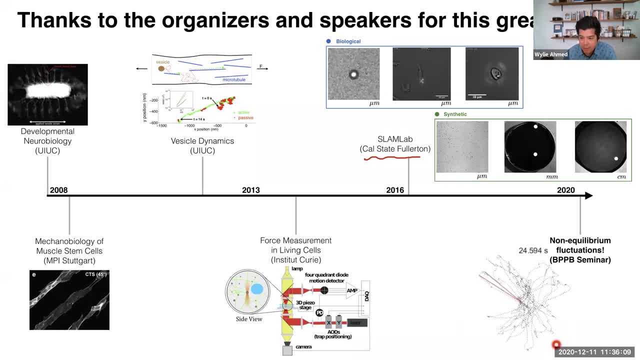 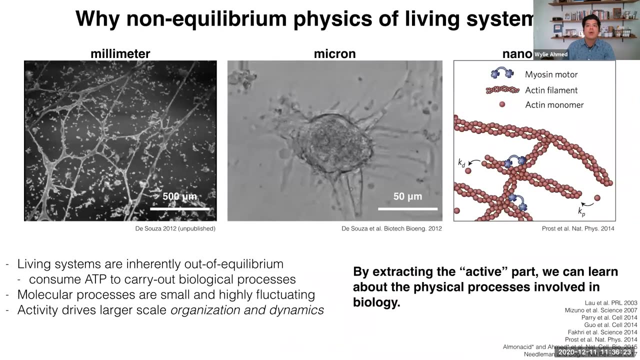 to talk to you about some non-equilibrium fluctuations, And this red thing here is a force vector that is measured by the optical tweezers for a Klamath-Amonis microswimmer stuck in the trap, And I'll talk a little about that today, as well as with theocytes. 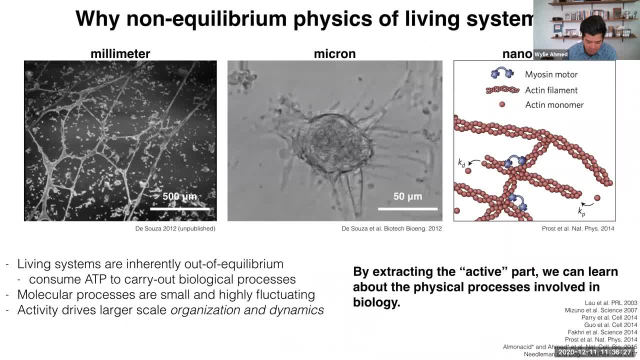 So I don't think that I need to motivate this very much for this audience. but the question of why non-equilibrium physics of living systems is so that we can get at the living aspects, so the active aspects, So at this nanometer scale. here we have these molecular motors And in this example 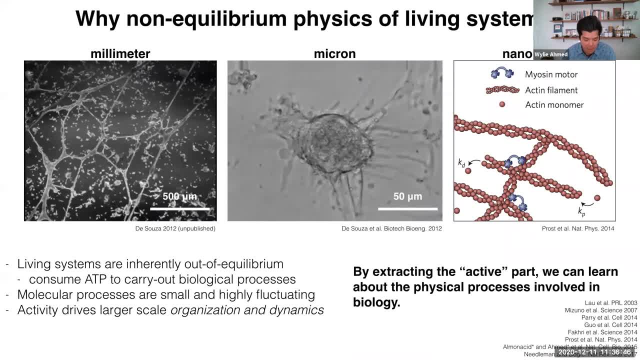 this is actin. Of course there's all kinds of things inside the cell that use energy, that consume ATP or other sources of fuel to drive the system out of equilibrium. This type of activity at this scale drives cellular activity, So this is a whole contracting cardiac. 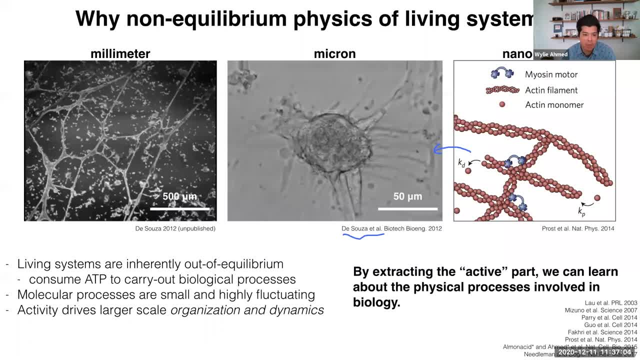 cell here which is beating, And if you leave that for long enough, you'll start to get larger scale organizations Like this, which is, millimeter scale organizations, And the idea is that if you don't have this activity, if you get rid of it, then you lose all of this interesting stuff. So what we're 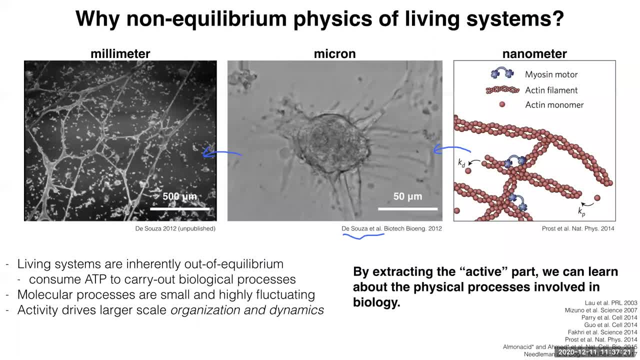 trying to do is focus on trying to extract what this activity is, to understand both the physics and the biology of these systems. That's really what drives what we do. There's many other groups working on this, of course, But so what we try to do is focus on extracting. 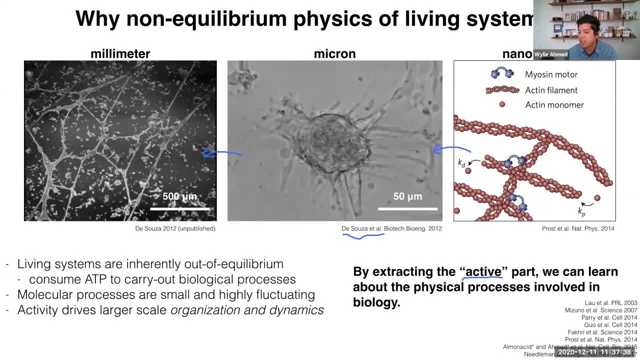 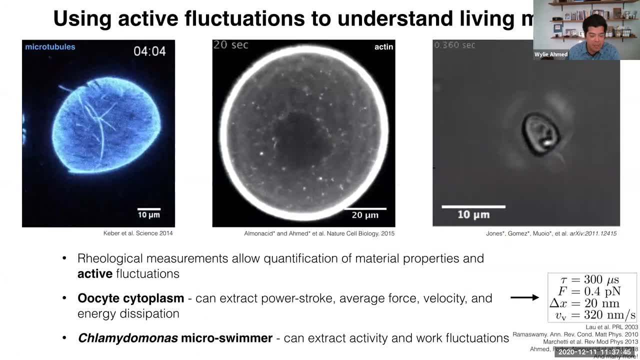 the non-equilibrium fluctuation, And by non-equilibrium I essentially just mean non-thermal. So we see this across all different scales, Like I just mentioned, this beautiful video on the left of microtubules and a liposome. This is not ours, But so, looking at the organization, 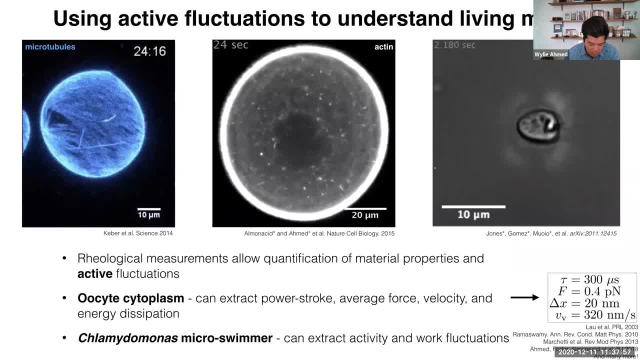 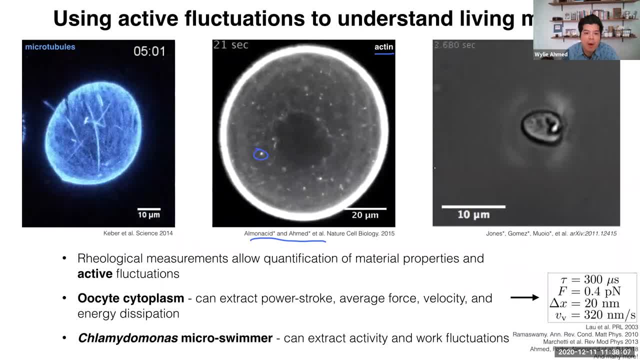 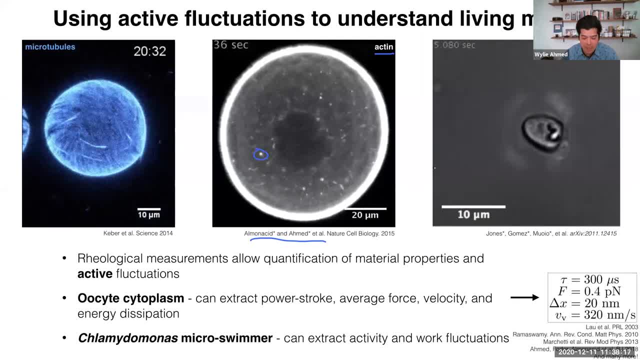 myosin V motors, And we're going to get to those details in a bit. And then we also apply similar techniques to understand the non-equilibrium fluctuations of entire organisms here. So this is our clamidomonas microswimmer stuck in the trap. You can see this diffraction. 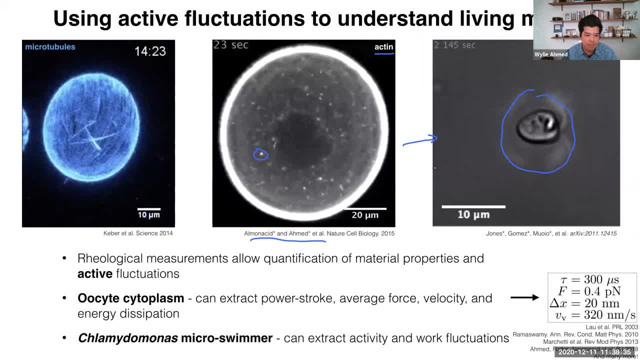 is coming from the laser. So we're hanging onto this little guy and you get some away, And what we do is we use rheological techniques, so what's called passive and active micro-rheology, to quantify the material properties and the active fluctuations. 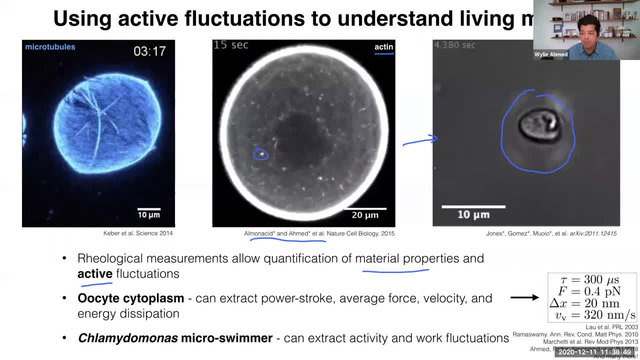 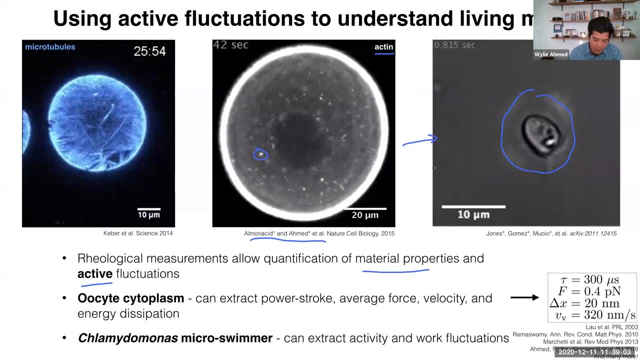 So most of the time our goal is not to quantify the material properties themselves- we're not so interested in material properties- but we characterize them so that we can know what fluctuations to expect at equilibrium. and then we can subtract those off and we can see what's left over, so we can see all the active fluctuations. 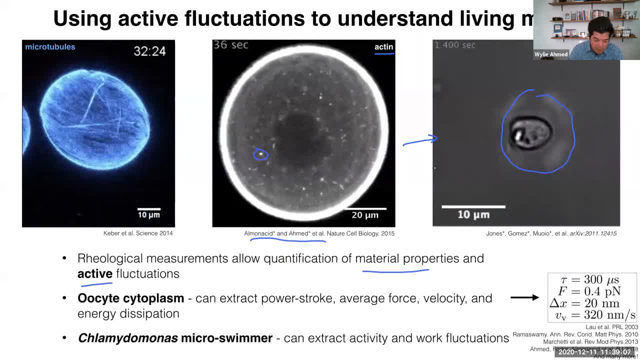 And applying this to these two systems, we've seen in the oocyte cytoplasm we can extract some kinetics which look like they're related to molecular motor kinetics, And then also at the climate of Monist microswimmer level we quantify the forces and we compare. 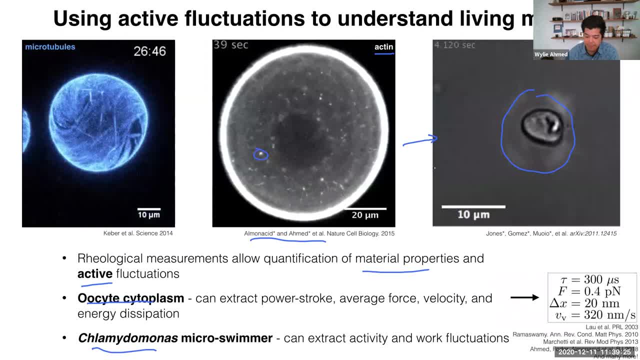 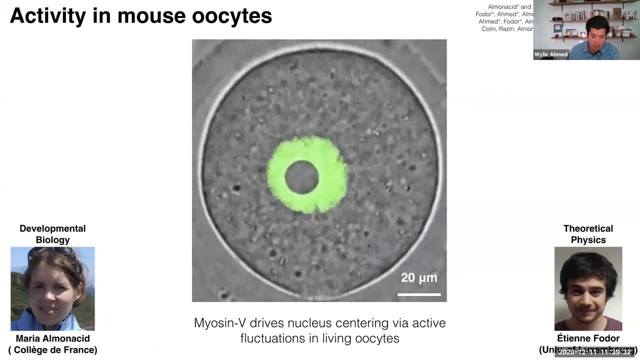 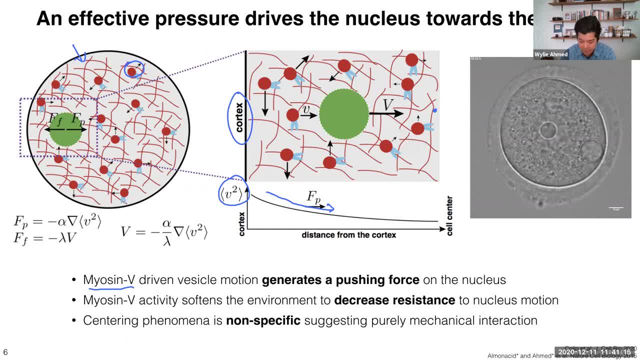 and surely there are a host of other things going on. But interestingly, more recently in Marie-Hélène's group they injected these oil droplets here and what they found was that anything that you'd inject in would get pushed to the center. So any mechanical object, this is just. 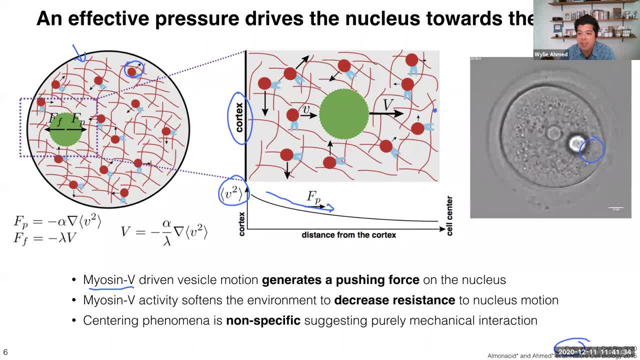 an inert oil droplet and as long as over a certain size. so there's some size exclusion. but this would get forced towards the center, And so this is kind of a general overall mechanism for- and I use the word nonspecific here- for centering any large objects in the cytoplasm. 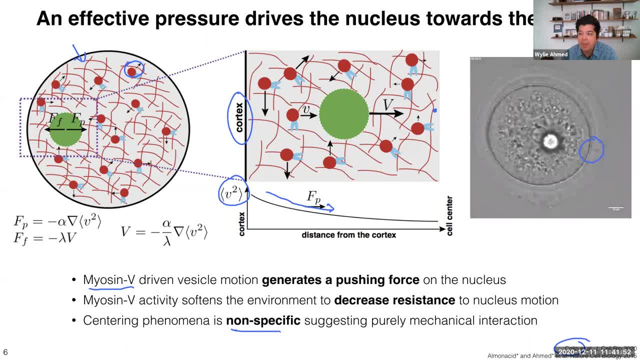 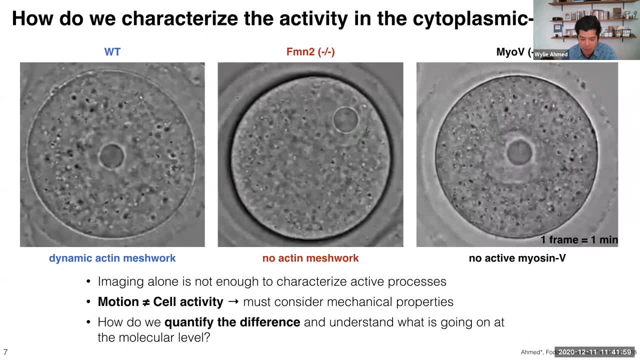 And so we found this really interesting, and what we wanted to do was to understand the cytoplasm itself and how the cytoplasm would drive this motion. So the question is, how do we characterize it? And the idea is here. I'll play this video. 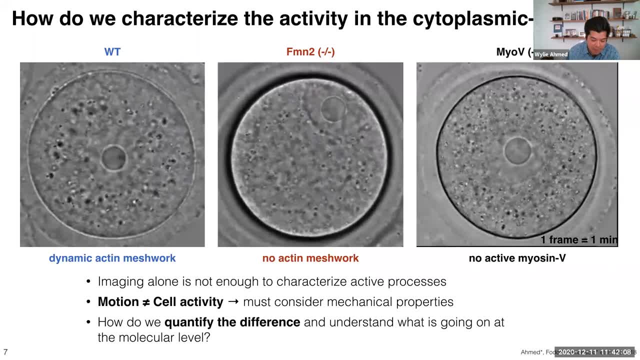 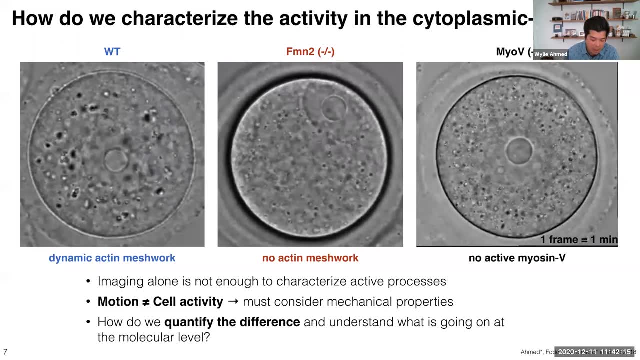 and in this video I want you to focus on the fluctuations of the vesicles in the background. Don't worry about where the nucleus is. so the this is the nucleus, but don't worry about where that is right now. Focus on all these fluctuations. 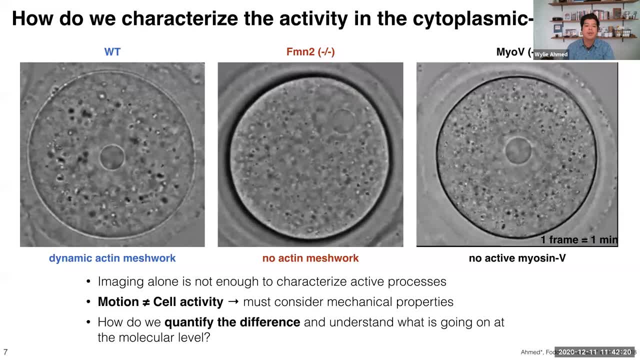 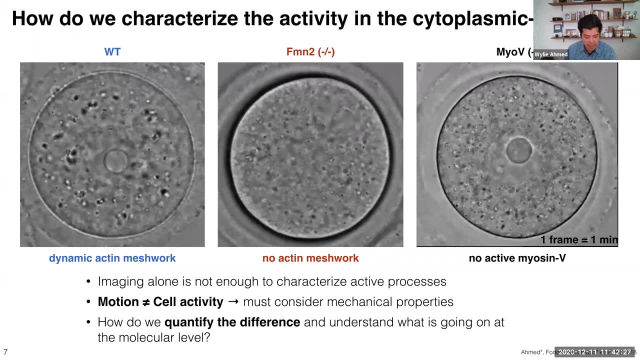 in the background here, And the idea is that imaging alone is not enough to characterize how active these systems are. right, Because on the left, here we have. so these are. this has a dynamic, active meshwork. here we got rid of the active meshwork and here there's no motors to. 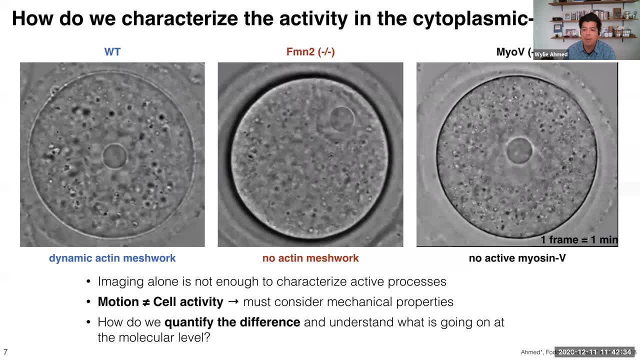 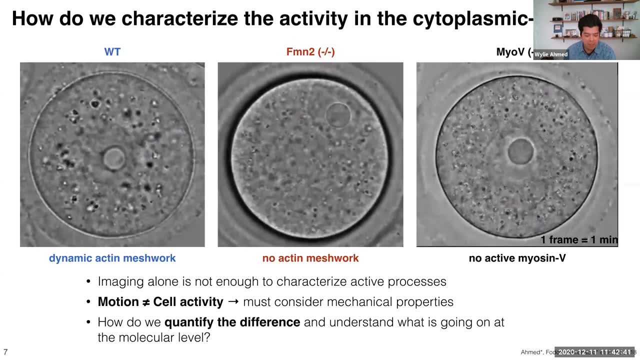 drive the network. So we know it's different levels of activity, Without priority. by looking at the videos we can't tell because in principle these could all be experiencing only thermal fluctuations. But this could be water, this could be glycerin and then this could be gelatin. 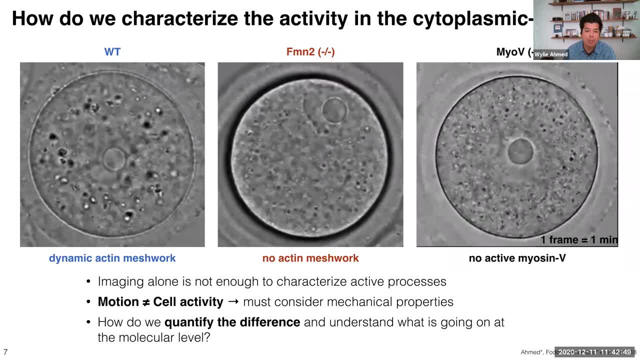 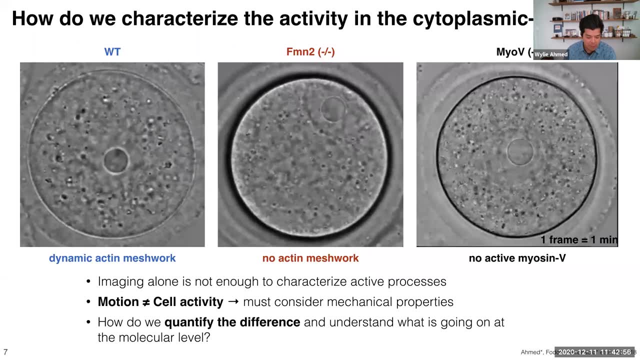 for instance. So what we need to do is to go in and actually measure what the mechanics are, not because we're super interested in the mechanics themselves, but then we would know what to expect from thermal fluctuations. So just the motion is not equivalent to cellular. 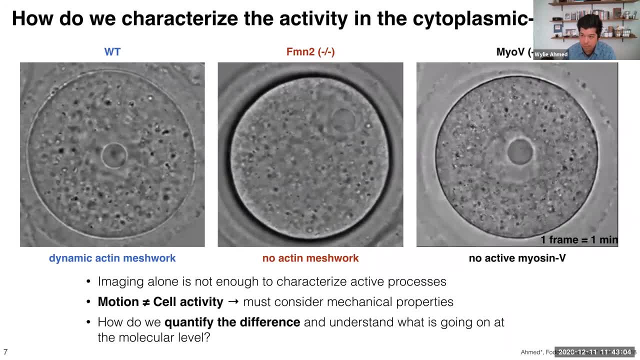 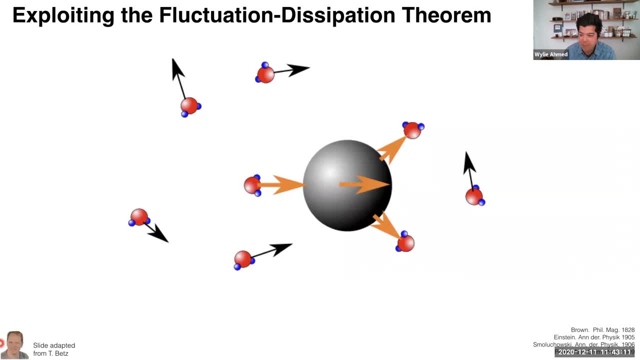 activity. so we need to go in and measure what's going on. The way that we do that is, we exploit the fluctuation dissipation theorem. I stole this from previous mentor, Timo, who's now in Göttingen, And the idea is now expect or think about a 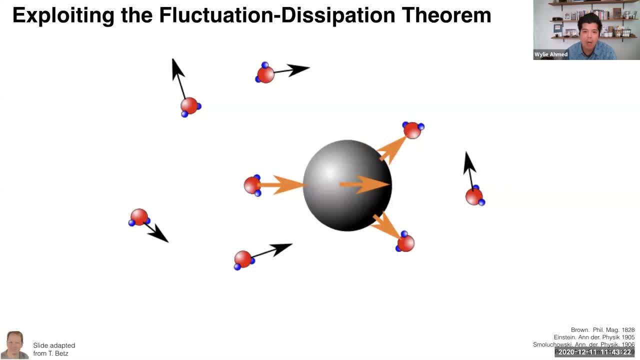 particle in thermal equilibrium. So this could be a dust particle in a glass of water or a colloid in a thermal bath, And the solvent molecules here are moving spontaneously. The solvent will hit your particle of interest. So this is the particle that you can see. There's a momentum transfer. 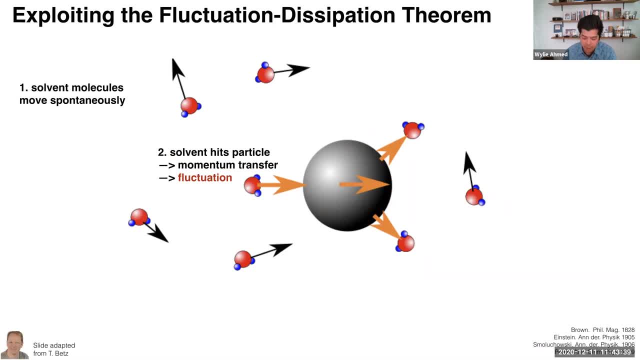 and that causes a fluctuation, And that fluctuation then makes this particle move through the solvent. There's momentum transfer as this particle bumps into the solvent molecules again and has to push them out of the way. So this is the dissipation part. So there's solvent particles hit your colloid, they cause a fluctuation, Your colloid. 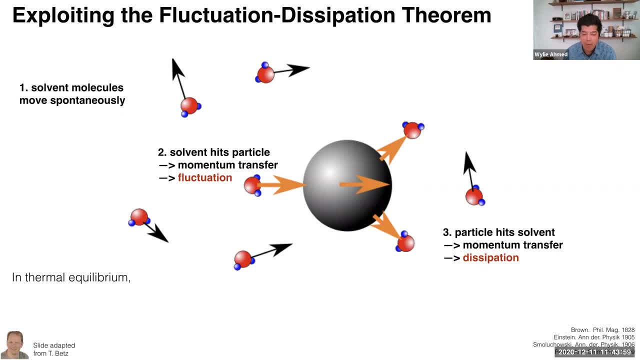 hits the rest of your solvent, which causes a dissipation Now in thermal equilibrium. this is well defined And it gives you a relationship between the energy transmitted by the solvents to create this fluctuation and the energy dissipated by the solvent during particle. 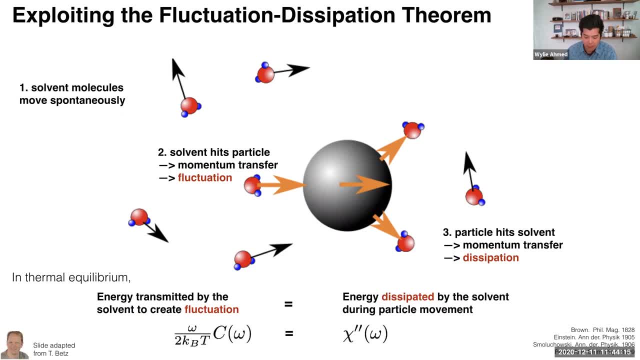 transfer. These two things are equivalent in thermal equilibrium And you can write this down: relating the imaginary part of the response function to the power spectrum of the position fluctuations, And this is a relation that's often used in passive micro-rheology, where you would 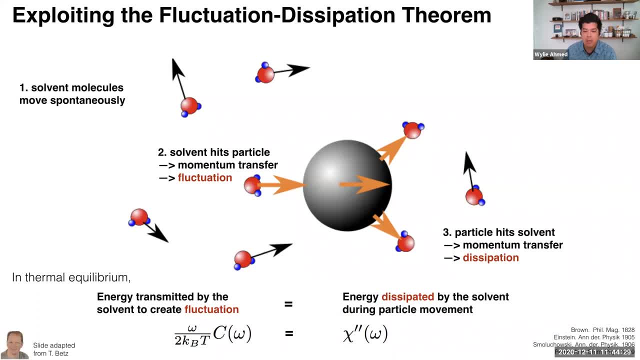 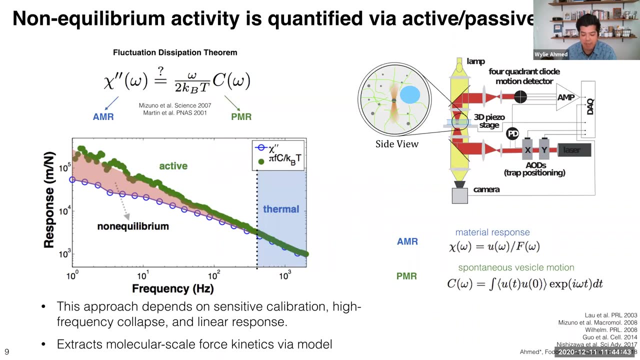 measure this and you would use this equivalency to calculate the response, And this is, of course, related to our familiar video of Brownian motion that we see here. So we use this technique and we use it in conjunction with active and passive micro-rheology to quantify the non-equilibrium. 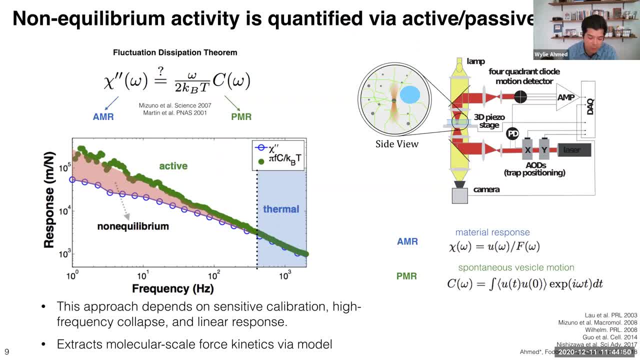 activity. So the way that we do that is we use this approach which has been used before, and we test essentially, I wouldn't say the validity, but how much the fluctuation dissipation theorem is not obeyed in these out-of-equilibrium systems. And the way that we do that is we measure. 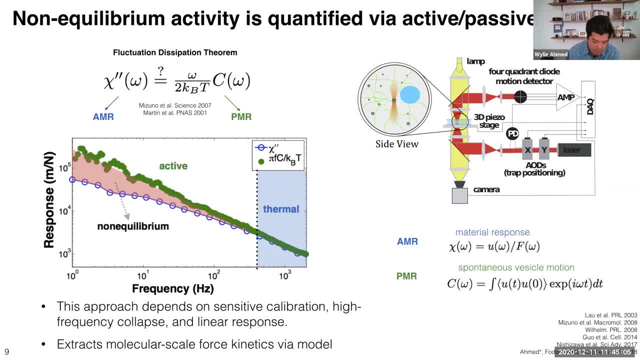 using. we measure the left side of this equation and the right side of this equation independently and then we see if they are equal. We use optical tweezers, which is shown over here. This is my terrible drawing of an oocyte. 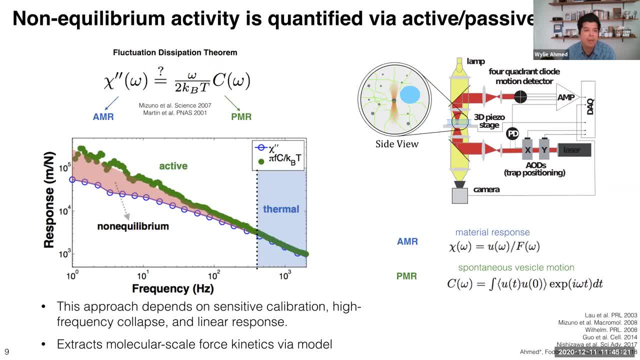 And so this is a typical optical tweezer system that's used by many other people, And the most important thing is that we can do active micro-rheology as well as passive micro-rheology, So we measure the two sides of this equation And, by the way, the way that we do that for active, 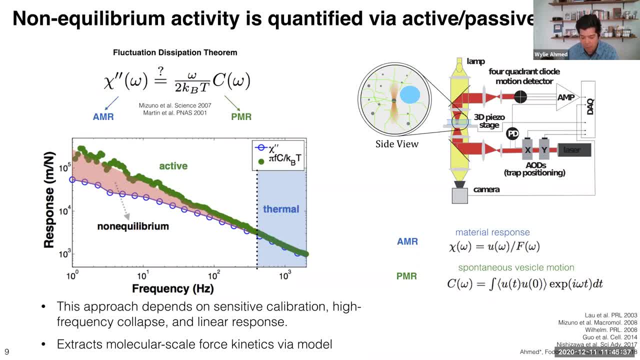 micro-rheology is. first measurement we do is a material response where we apply some displacement, Actually we measure the force, And then from that we can get the full response function. So not just the imaginary part, but we can get the full response function And then as a separate measurement we do. 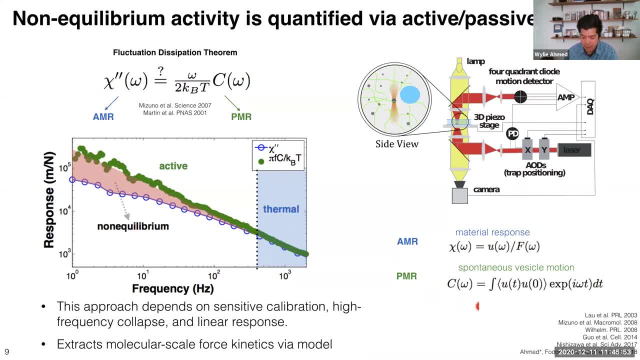 we measure the spontaneous fluctuations of the vessel and look at the power spectrum of that, And that's essentially related to passive micro-rheology. So here this: these two things are plotted in this plot here, And what we see is that the response function gives us this lower line. 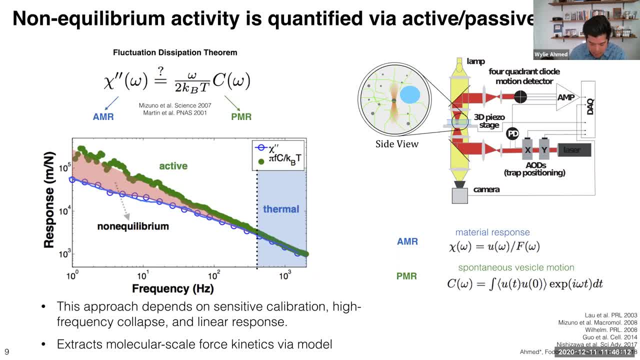 here. And then the active part, which is the spontaneous motion, gives us this upper line here, And what we use is: we try to take this area in between, extract this information and see what that can tell us about the system. So that's mainly what we're interested in here. So there's. 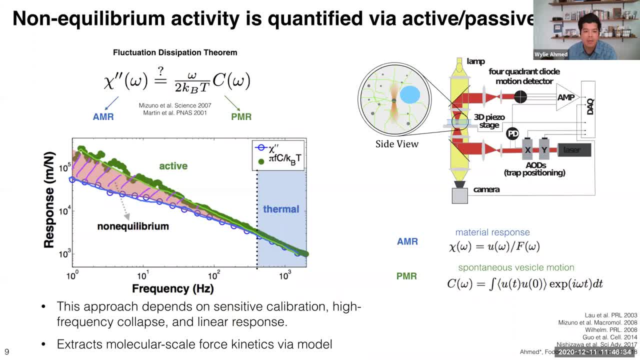 all kinds of calibration involved in this. I'm happy to answer questions about that later, But what we see is that at high frequencies these two things equal each other, And at lower frequencies they don't. So FDT is violated and we use this information to try to extract something from the system. 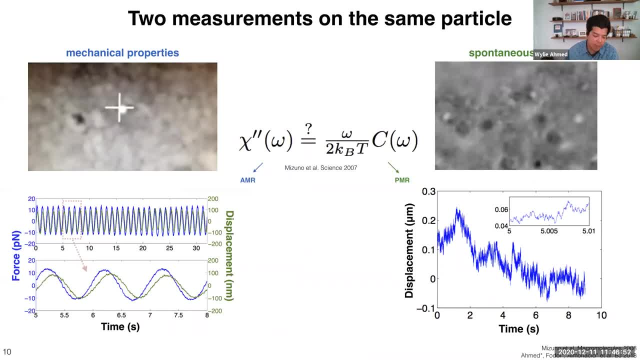 So, just to drive that point home, we do two measurements on the exact same particle. So here we have this oscillating particle which we we're trapping and replying in displacement. From that we can get the response function And then separately we measure the spontaneous. 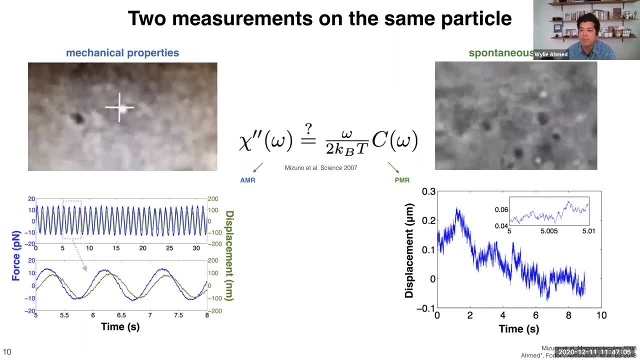 fluctuations of a particle. So we calculate the left and the right side independently for the same particle in the same situation. Of course they can't be done at the same time, but we do them right after And we can switch them to make sure that doesn't make a difference which one we do first. 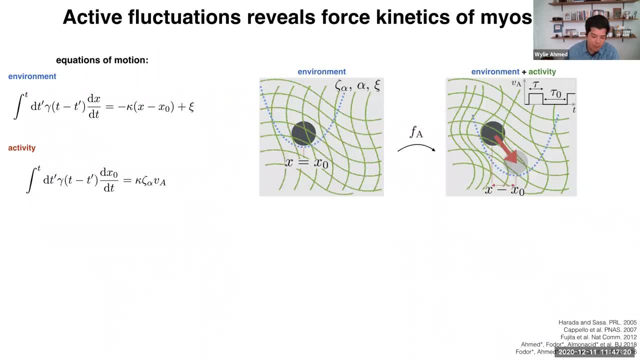 So to make any sense of this, then we turn to modeling, then to make any sense of our measurement, So then we, we model the environment. So this is the cytoplasm here As a viscoelastic environment that is characterized by some viscoelastic memory. 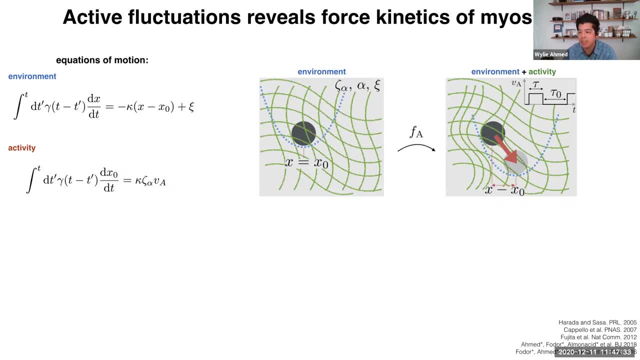 kernel. it's experiencing some local trappings and local caging stuck in the cytoplasm And of course there's thermal fluctuations. And then we say we add an active force to this. which, this active force, we use the simplest model for active force to think of, which is essentially telegraph noise. 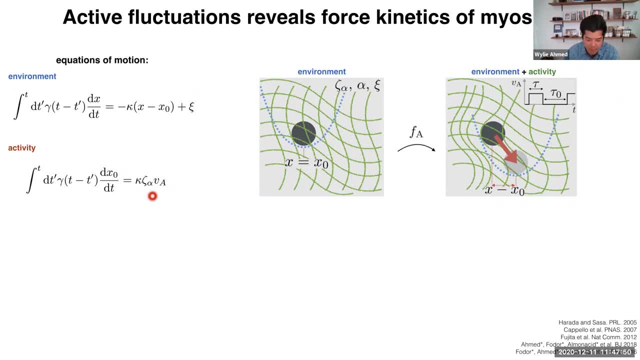 And then we say that this active force comes along, which is the right side of this equation. here This is just simply force balance. The force comes along and rearranges the environment and drives your particle to new locations. So, from this approach, 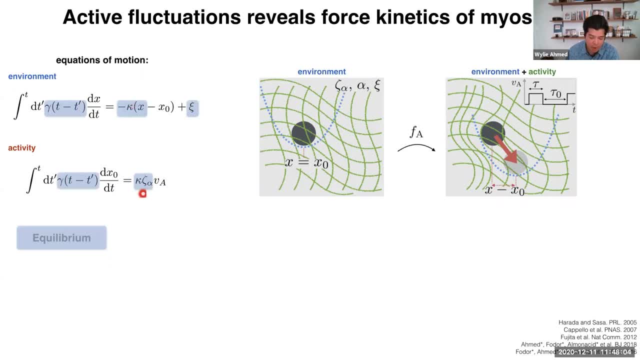 you have these equilibrium parameters here, So all of these can be measured from your active microbiology. So we're getting the response function from the system, And then we have these active parts here which we're extracting from the model. so this is what we don't know. 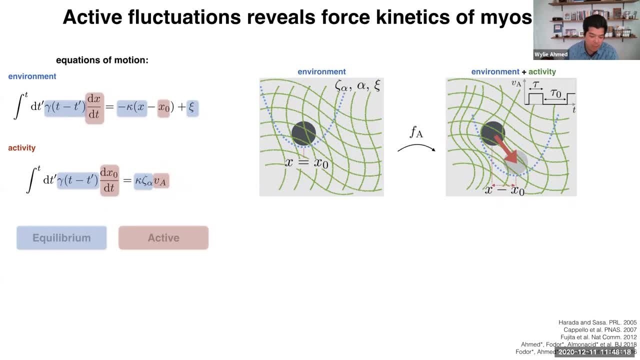 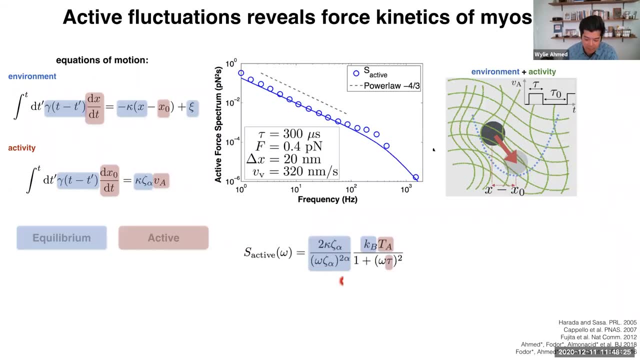 this is some stochastic process here, and from these two coupled equations- so they're coupled because this goes in there- we can derive the active force spectrum here. so here we have again these blue things or equilibrium properties. so we have two parameters left over and in actuality, 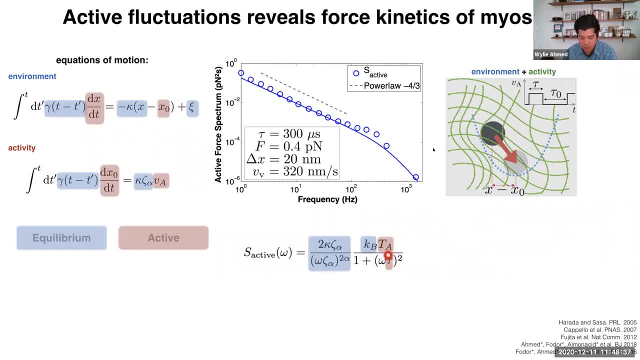 we've already determined one of these, but that's not important right now. but so we have these two fitting parameters, you could say, to fit our active force spectrum, where the data points are. these circles are our measurements, and then this curve here represents this line. and when we do, 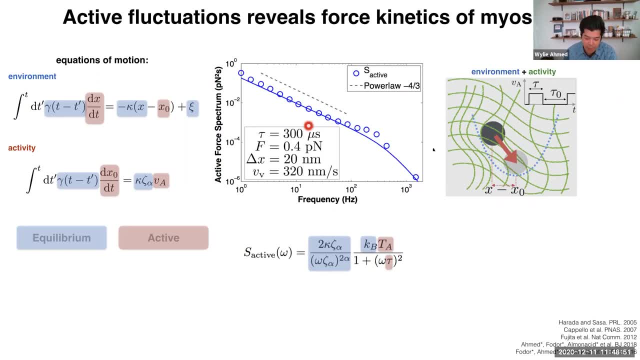 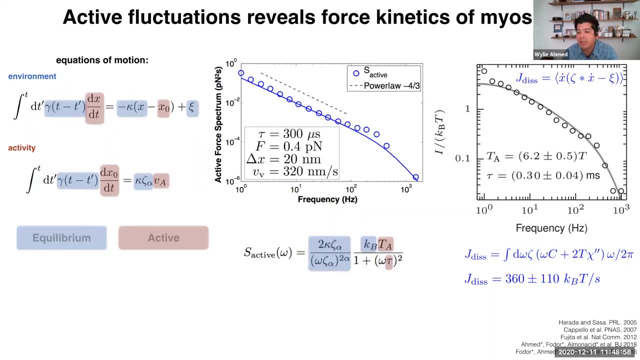 this fitting. we extract these parameters here and and what we can see from these parameters is that they tend to line up with what's seen for myosin 5 in single molecule measurements. so we can't verify that of course these are single molecule measurements because we're just doing measurements. 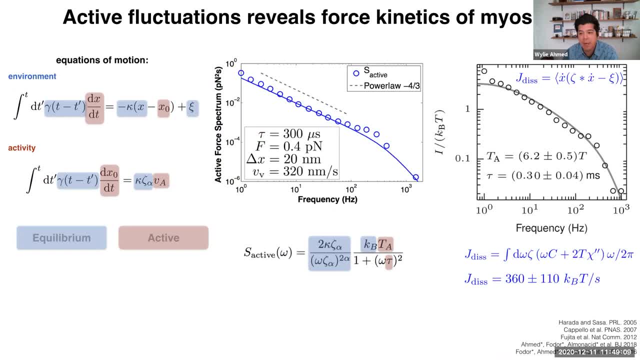 in living cells. but these kinetics agree with what's expected from myosin 5.. and there's another way to write this: to look at this information, which is the Harada-Sasa quality, which I won't go into the details of, but essentially this is the amount of energy dissipated. and if you integrate this, 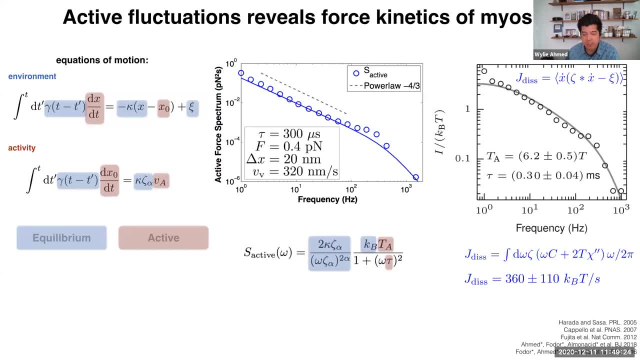 you can estimate the amount of energy dissipated in this process, which is essentially just a measure of the violation of FGT, and here we get this number here, which corresponds to about 20 motors. so it seems like we have roughly 20 motors in the area of these vesicles that are driving. 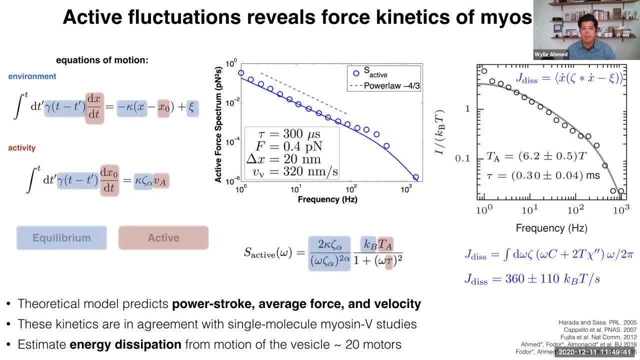 their motion. that's an estimate that we haven't yet been able to verify, but it seems it's, at least it's a reasonable number, and these other kinetics also correspond to what happens for very close numbers, for single myosin- 5 actually. but so, using this, all we've done is doing active and passive. 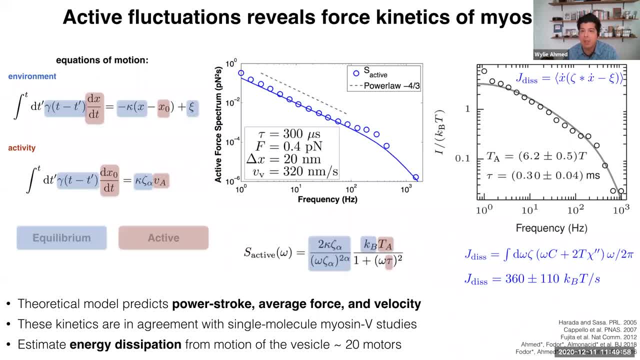 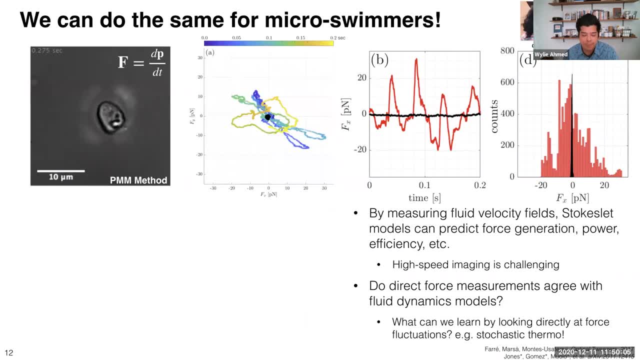 microbiology to extract what looks like kinetics and what's happening at close to the molecular scale, and so in my lab what we did is we tried to apply this technique to another system here, which is these microswimmers. so there's Clamidomonas, and again for the students, I want to point out that 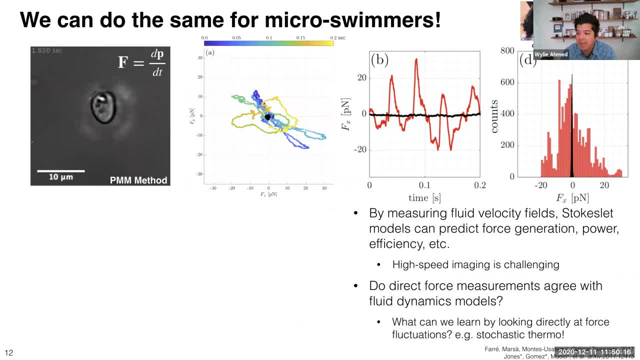 I never worked with Clamidomonas before. I still don't really know anything about them, but so what we? the way that this worked was: I was looking, I set up my lab, I was looking for something to measure, so I went to the arboretum and pulled stuff out of the pond, and then we found 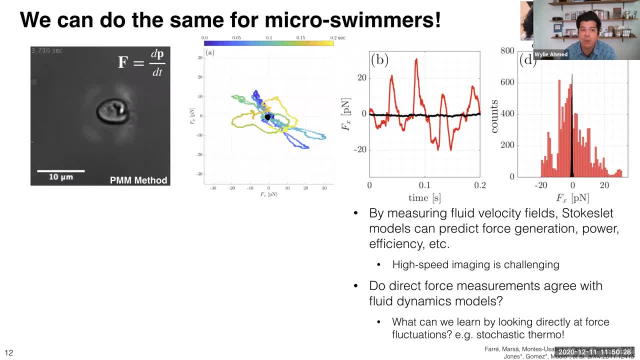 out. I didn't know what these things were. I asked somebody else and then found out that we could start doing controlled experiments and actually ordering them. so I don't claim to be to know anything about algae or Clamidomonas biology, but these micro swimmers are the ones that are going to 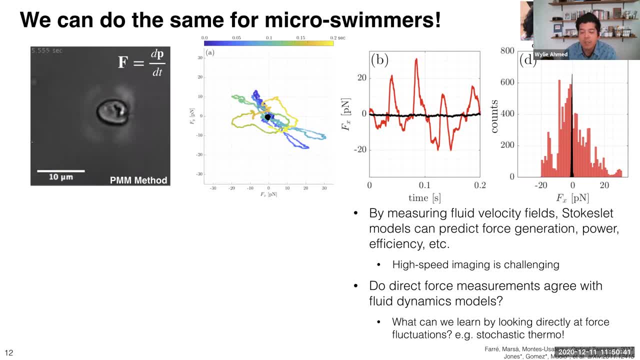 be able to do that, and so these are our active particles that are stuck in our trap, and we measure them. so here we use a different technique to measure the forces. again, I'm happy to answer questions about that later- but we use what's called the photon momentum method. 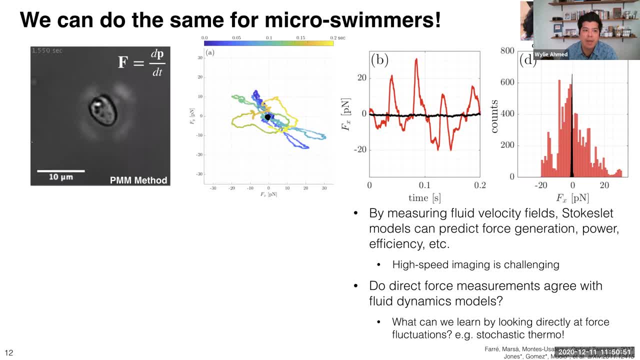 we measure the change in the light momentum directly. the reason why we have to do that is because we don't know the index of refraction or the size or anything like that of the Clamidomonas. so to get quantitative force measurements, this is the only way that I'm aware of of how to do it. 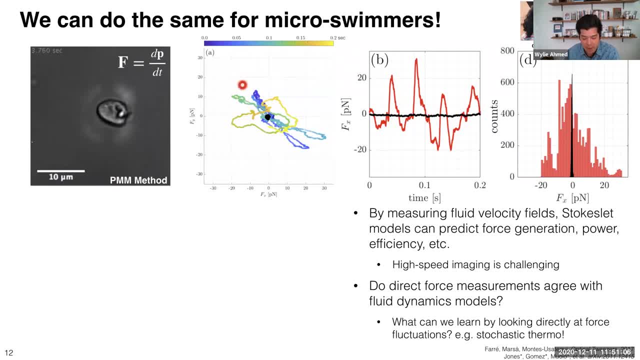 and so we measure the force fluctuations of the function of time. we can get these very high intensification force trajectories here. so, by the way, this, this black center here is and this black data here is for a thermal particle and the rest of it is very climbing. this is work done by my 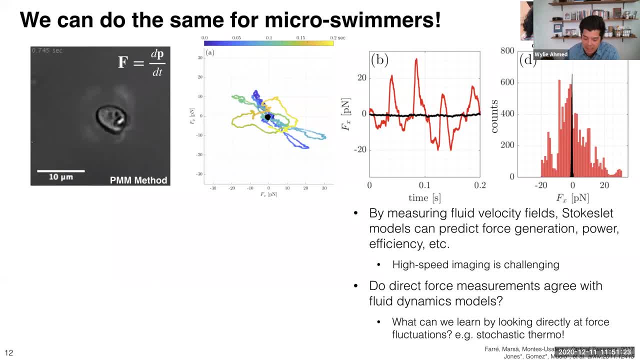 students here, by the way. so Corbin did a lot of these measurements, and then the idea is that we want to compare the direct force measurements to what's been seen before in these in the fluid dynamic states, because there's been a host of fluid studies done that have been really beautiful. 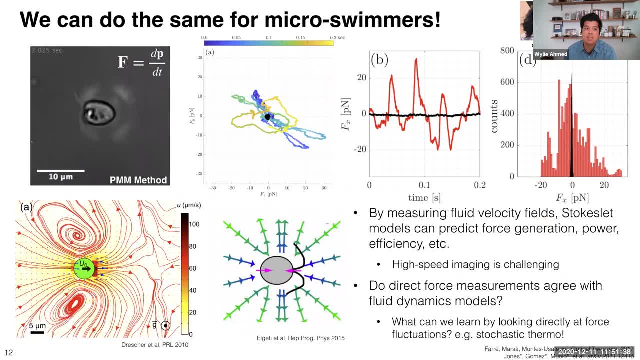 and what they do is they look at the fields that these swimmers generate And they use models- often steps with models- to predict the force generation and the power and the efficiency. These experiments are fantastic. They're also very challenging And high-speed imaging is also challenging to extract the very 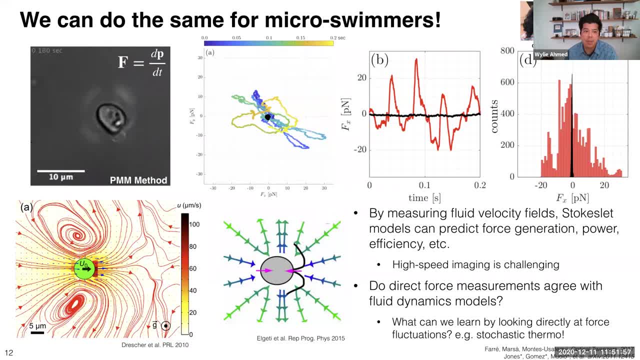 rapid fluctuations And so, since we're mainly interested in 90-kilogram fluctuations in my group, the fast timescale fluctuations- we decided to apply these optical tweezers And our question was: if we measure the force directly, do our results agree with what happens if you look at? 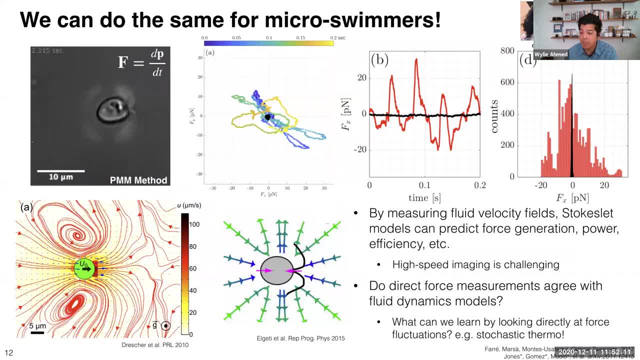 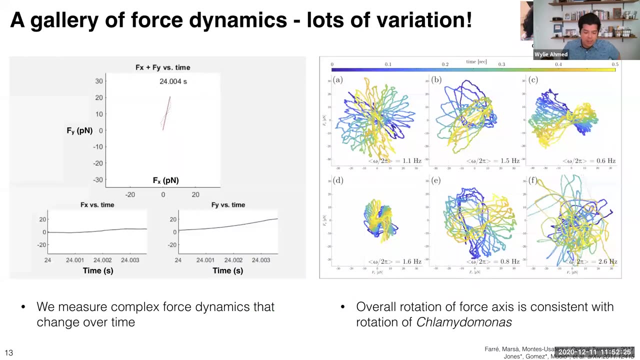 the fluid dynamics, And luckily they do for the most part, So I'm very happy. I had no idea if that was going to work or not, But so by directly measuring the forces we get a lot of the same quantities, And that's what I'm going to tell you about today. So here, the first thing we noticed. 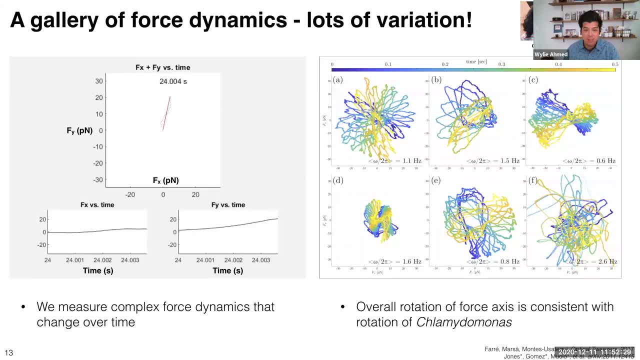 was that there's lots of variation in these force fluctuations. So on the left you're going to see an example. This is an example of a force fluctuation, And this is an example of a force fluctuation. And this is an example of a force fluctuation, And this is an example of a force. 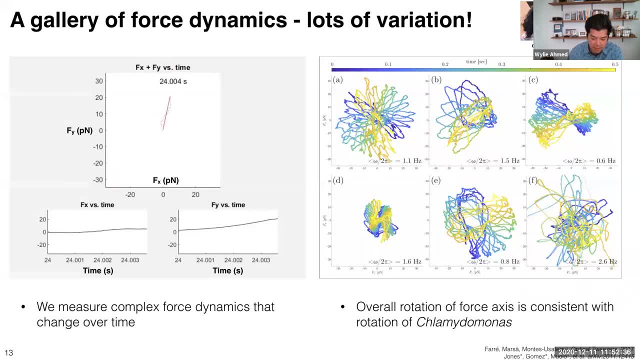 This is the force vector here. as a function of time And as we play it, you're going to see these fluctuations. So there's a large oscillation, It's a noisy oscillation And it also has this rotation. So we see that very complex dynamics And we also see many different patterns. So we 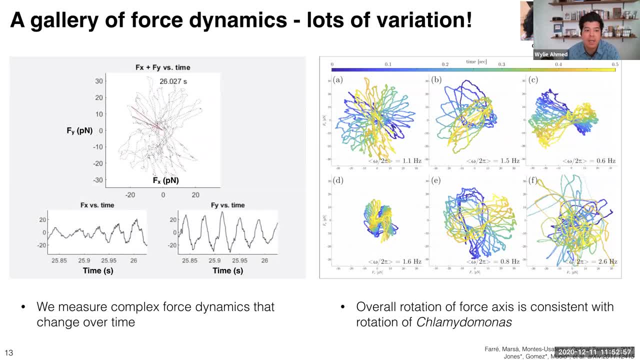 see different patterns, transitions between these patterns and identifiable groups, which would be super cool to apply something like machine learning to understand these At this point. Corbin was the machine and he used his eye to identify these different types of phases, And we're 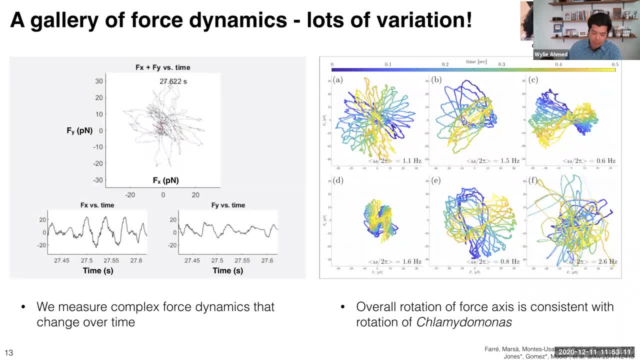 still looking into trying to understand the transitions between them, But what we see, at least at first glance, is that if we look at how this force vector is oscillating back and forth and how that kind of rotates as a function of time, then we get this rotation here of the swimmers, which is 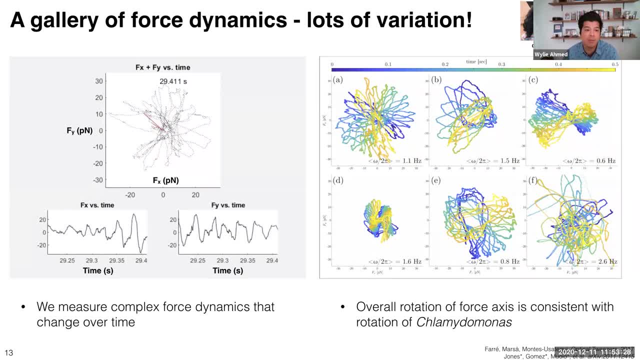 also consistent with what people have seen in the helical swimming of the clamutes, which was satisfying, because this is a lot of time And we're still looking into trying to understand the oscillations, So this is a lot easier for us to do. Essentially, we measure a force signal and 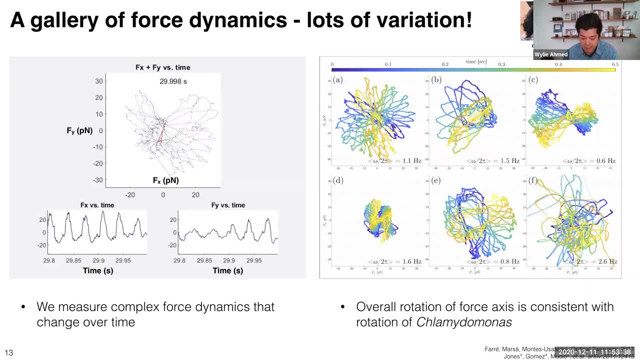 then we just take the spectrogram of it And you can see that there's an oscillation of these frequencies here. The nice thing about this is you can do a point-by-point measurement. So every swimmer, you can characterize this and you can characterize as a function of time. So, as I said, 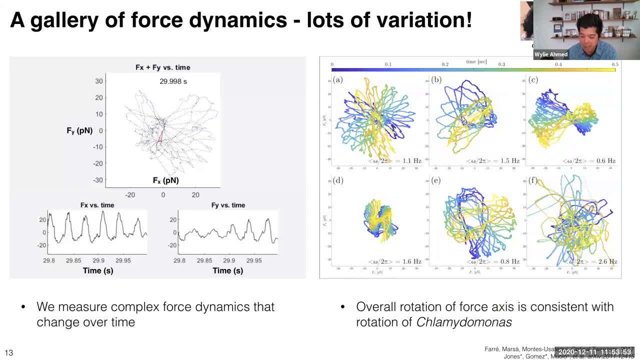 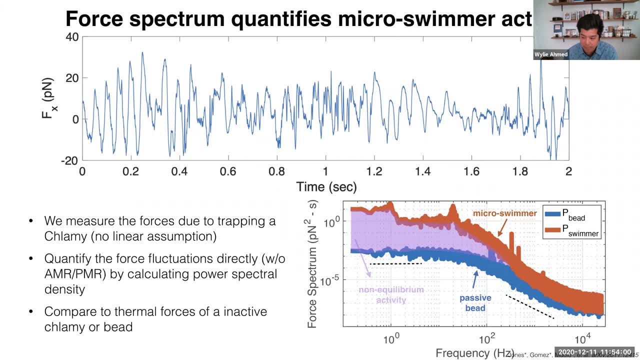 we don't really know what to do with this information yet, because we're still looking for ways to characterize this. So we go back and do what we know how to do, which is we look at the force fluctuations and we calculate the power spectrum of them. 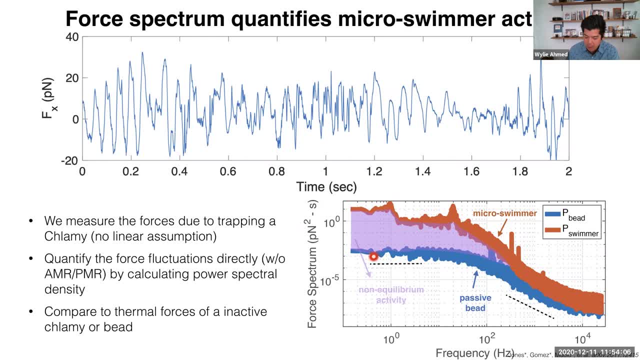 So here we see this is. you could imagine this to be the power spectrum of a passive bead or a dead swimmer. They look very much the same. And then the power spectrum of a living swimmer. here we have this information here And again, we want to extract this information to try to understand what's. 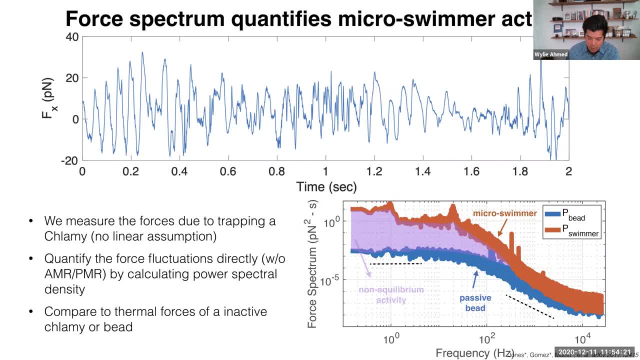 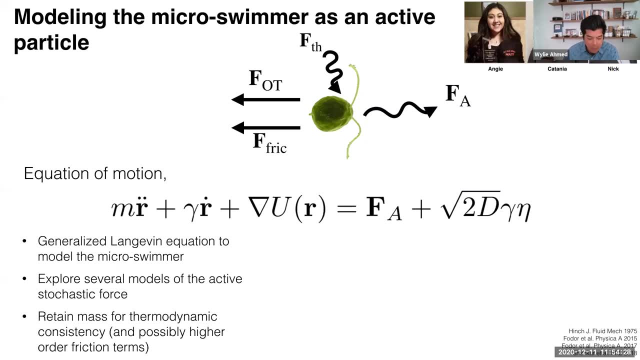 going on. So, of course, we again turn to modeling, and this is in collaboration with some colleagues in math, And so the idea is to include inertia, and that's actually, you know, that's what we're doing, largely because we want to look across certain scales. So, in this case, what I'm going to 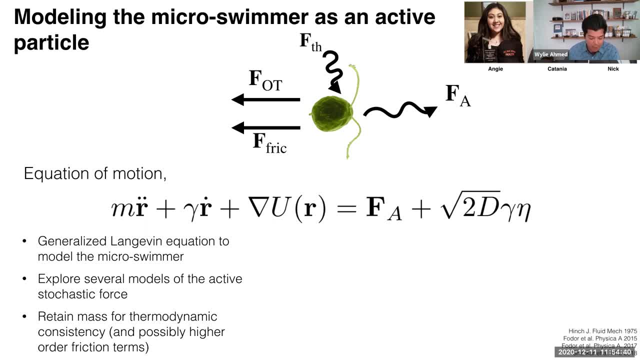 tell you about today is we do throw out the inertia for the microscopic scale stuff, But the idea is to explore a couple of different models. So some of you may be familiar with these two models here, which are very common in active matter or driven particle dynamics. And then we also add one 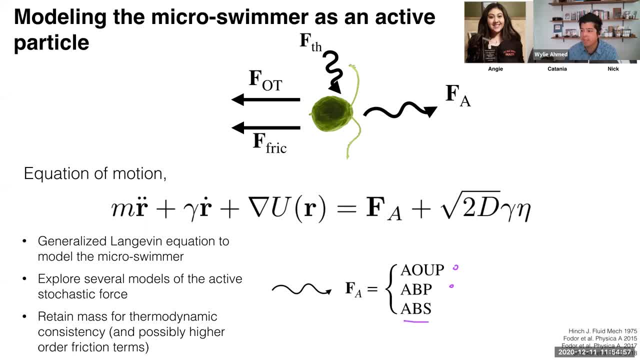 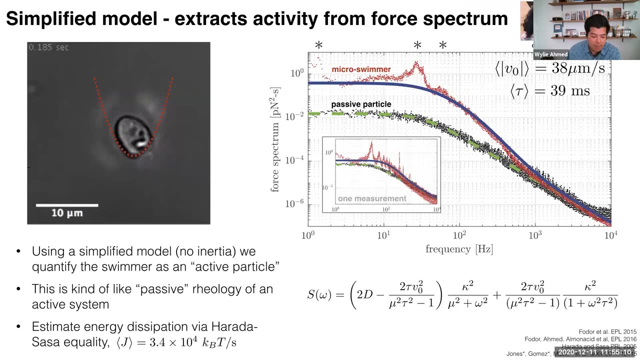 at least in simulations for now- which is an active beading swimmer, because it's pretty obvious that the climate is swimming, And we take this approach as a single particle approach, again to see how well it aligns with the fluid dynamics approach, which looks at the entire flow field. So by 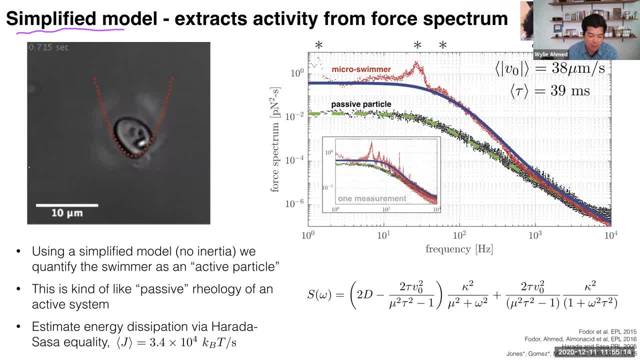 simplified model. here I mean that we throw out inertia again. So we have our little clammy in the trap And what we do is we calculate the force spectrum again. So then we have this lower curve here, which is a passive particle, And then this data up here which, notably, the model does not. 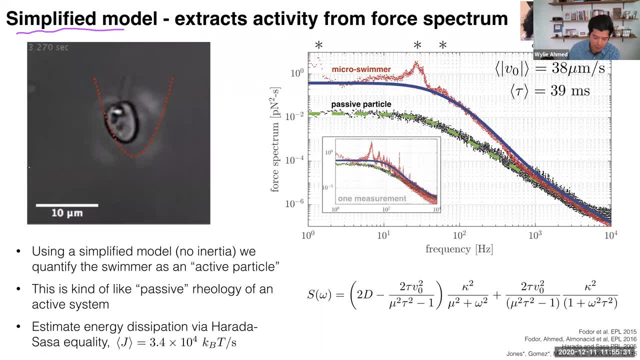 capture these peaks- but I'll talk about that in a second- And so we can look at these two models here. We can derive our power spectrum from our equations of motion, And I think of this as kind of like a passive rheology of an active system. So luckily we know what the properties would be in. 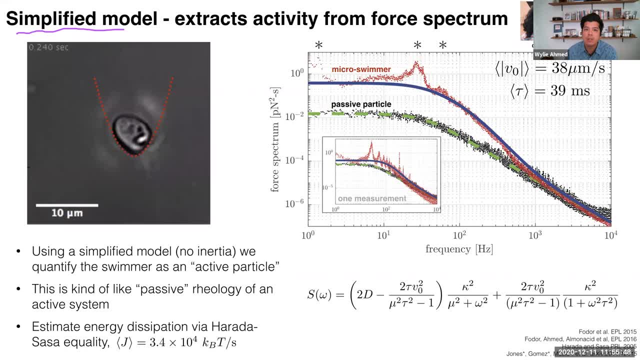 the thermal fluctuations case which is here, And then we use this rheology to extract only the activity. So we're interested again in all the stuff in between. So we fit our equation here, where here we have again all the equilibrium properties. So then everything in blue is already. 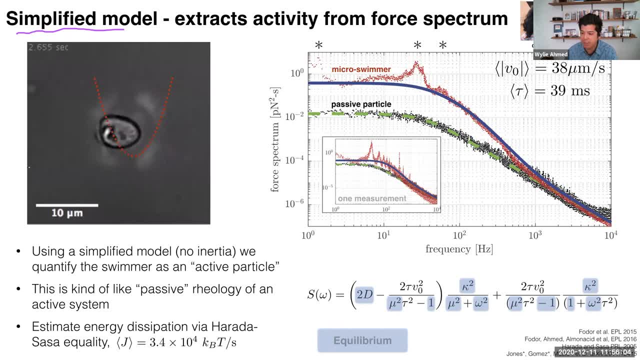 determined by our trap And water, because these climates are just swimming in water. And then we're left over with these active parameters, which really is just tau and V0. So we fit our tau and V0 to our power spectrum. here We extract an average V0, which is the average velocity of our active force. 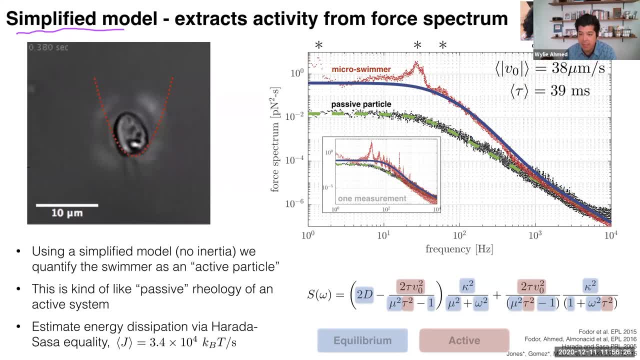 which is 38 microns per second, and then a tau of 39 milliseconds. It's a little bit harder to interpret these in the context of the swimmer because they're varying a lot, But we can see that they're varying a lot over time, But this is significantly lower than you would expect. 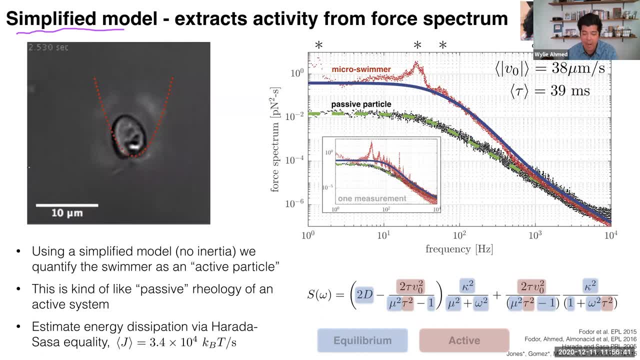 for a single swimming in climate months. But that's because this is also an average over all particles that are also or particles, clannings, that are also sometimes quiescent. They're not actually swimming. From these we can do a similar calculation where we estimate the energy. 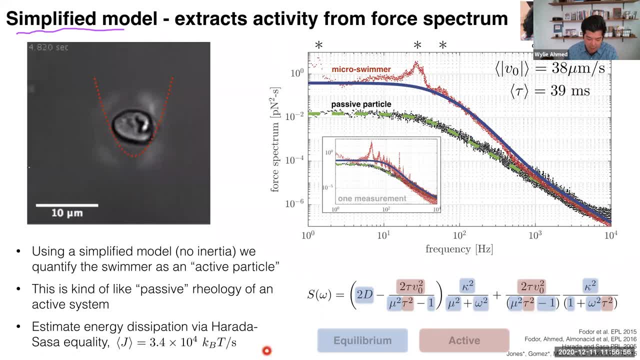 dissipated from the Herata-Sausse quality. And we get this number here, which may not mean much at first glance because I have no context for it, But it's moving. This is about 0.1 femtowatts. 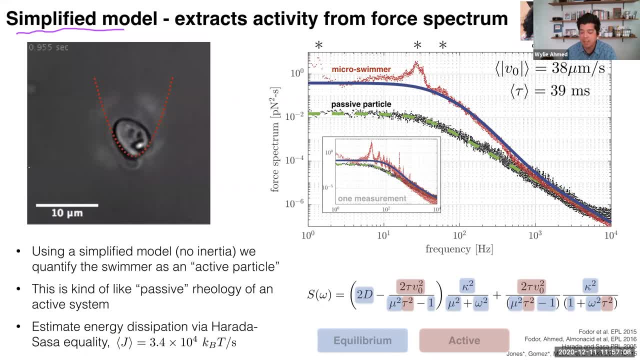 which is smaller than one would expect for a swimming clammy from the fluid dynamic studies. So then, what we did was we went to go like an individual clammy now. So here, looking at the individual trajectories. so from these trajectories I'm plotting the time course of what's happening on the left. 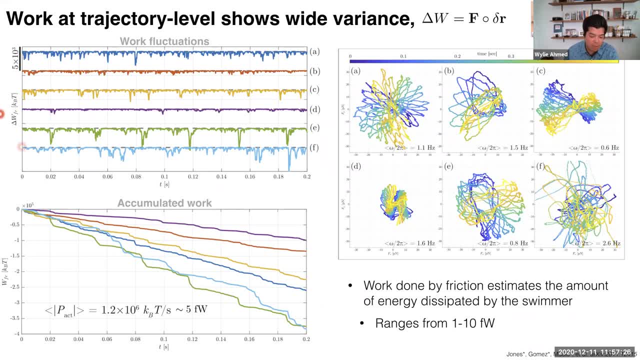 And we can see that there's lots of variation. So this is the work, fluctuations, and the work done by friction or heat, you could say, And then this is the integral of that, so the accumulated work. So, really, all I want to say about this slide is that, looking at these, 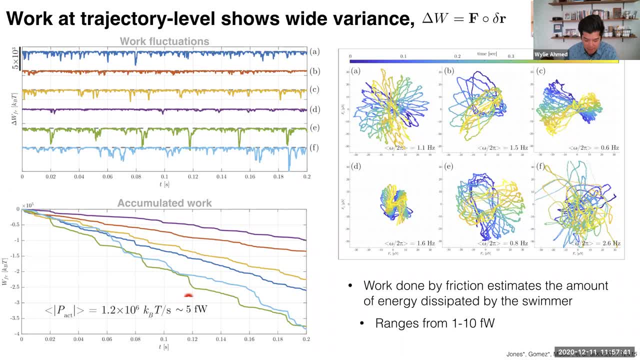 different clammies. here you can see very different amounts of accumulated work or heat generation, you could say. And so this allows us a way to, for instance, look at, if we look at D here, this, this is clearly less active and that's this one here. And then, if we look at 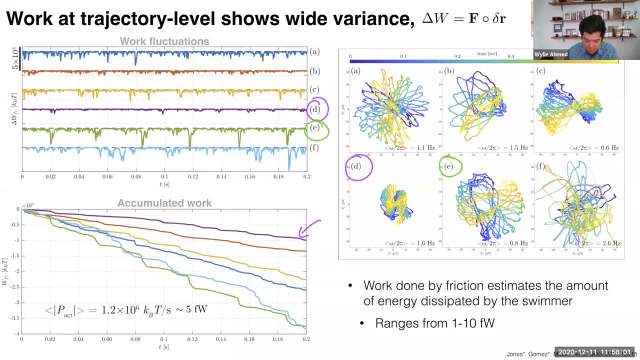 let's see E, this one that's more active, that's this one, And then that's this curve here. So this gives us a way to characterize the individual energy dissipated by these swimmers. where here this is. this was about, I think, one femtowatt or so, and this one is about 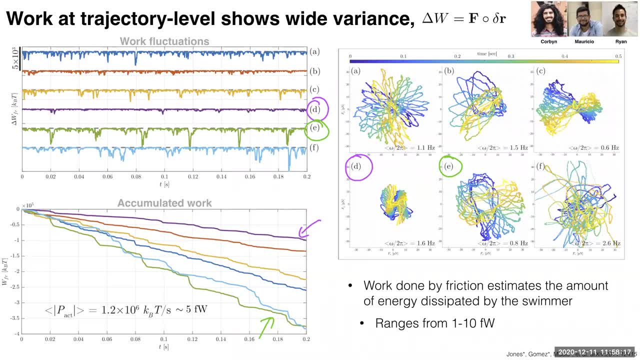 10 femtowatts, So we can start to look at the variation between them. So, Wiley, you have three minutes left. Okay, great, Thank you. So we see this range here of one to 10 femtowatts, And so what we'd like to. 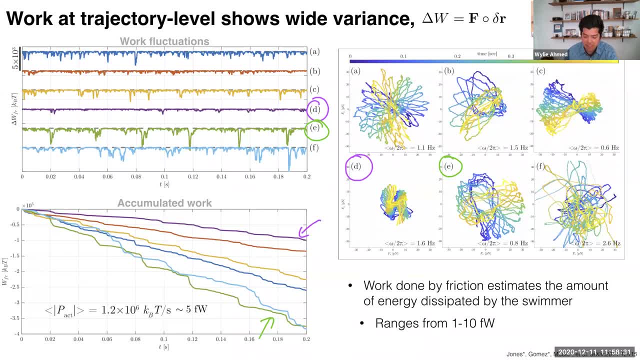 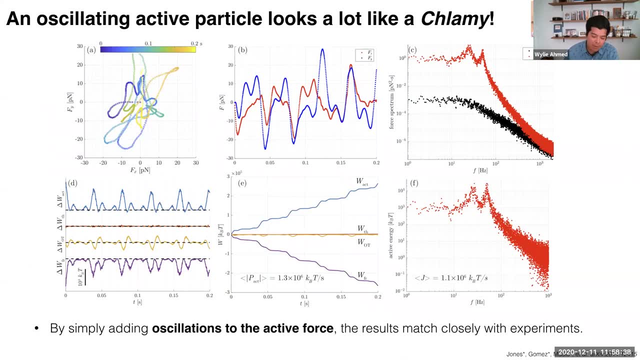 do next is to kind of characterize how they transition between these different states and see if we can find any patterns there and see how these, these clammies are using their energy, And to go back for a second to to look at how our model did not capture those. 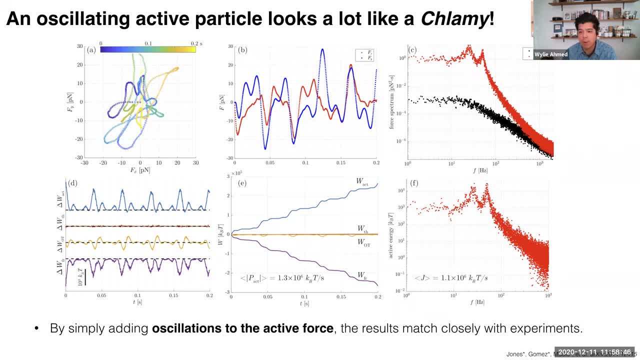 local oscillations And certainly, if you look at the trajectory level dynamics also. our model was not predicting what it looked like, So we went back and all we did- we did the simplest thing we could think of, which is we add the oscillations to this active force. 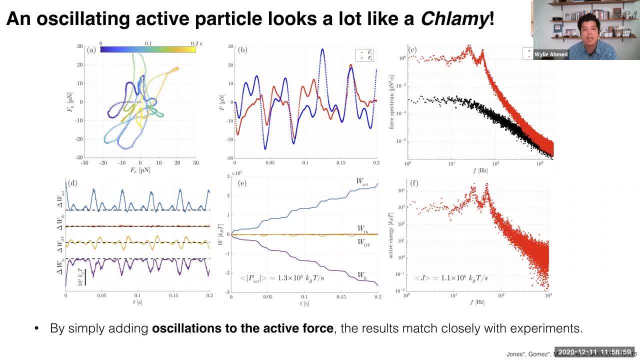 And so by adding oscillations I mean simply adding a sinusoid onto the active Brownian particle model. So when we do that naively, we get trajectories that look a lot like the ones you see with the clammies. We have these kinds of rosette shapes. 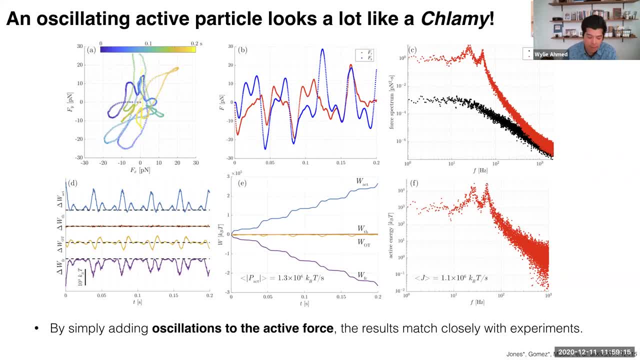 and then they're. they're spinning about the origin as a function of time. Of course, we see oscillations in our forces, but now we get these peaks in both our higher spectrum and our dissipation spectrum, which line up pretty well with at least the very active swim. 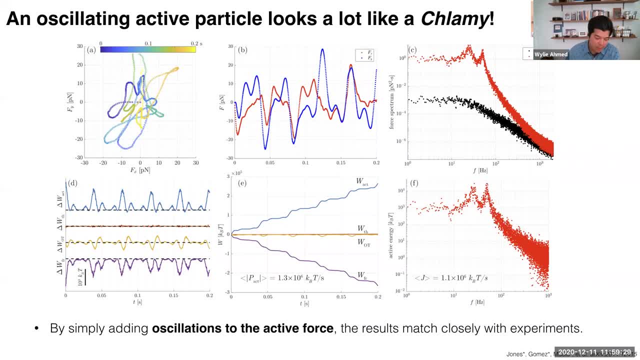 is because here we're simulating very active summer. Similarly, the, the fluctuations in the and the work and the energy dissipated as a function of time, as well as the energy dissipated from the route of saucer, relation lines up surprisingly well. So I'm actually 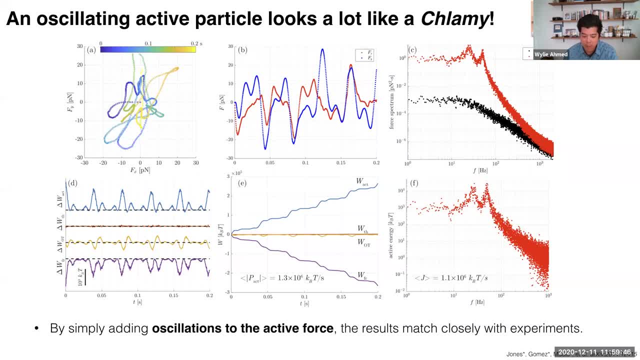 pretty surprised that this works so well. So we're not quite sure why it works so well, because all we did was very naively add this oscillation of active force. but but it gives us some hope for being able to explore some things computationally, to look at trajectory level. 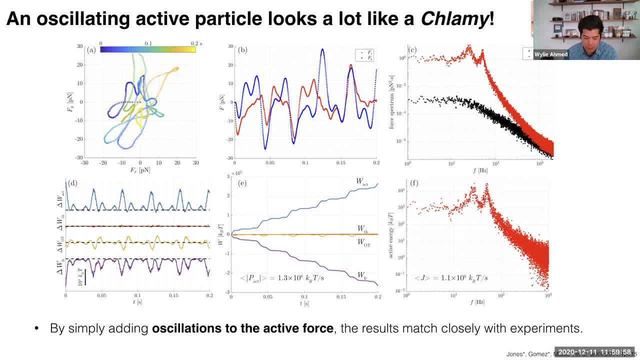 dynamics, which is something we're working on right now. So I'm going to go ahead and show you some of the things that we're very interested in. So, with that, I want to say that our take home message is really that we're using 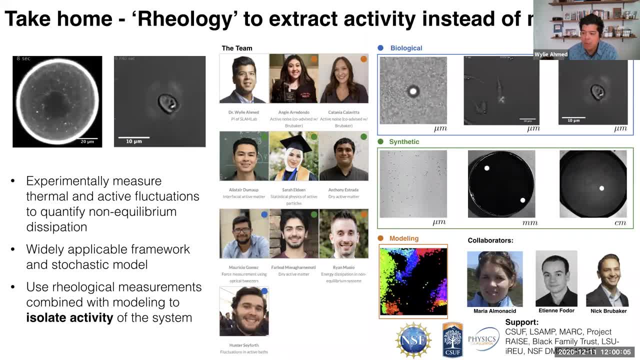 rheology to try to track activity instead of mechanics. So of course, we do the reality to determine the mechanics, And then what we really do is subtract all that out to try to get at only the activity. And so this has been. this is my army of students here, And so they're working. 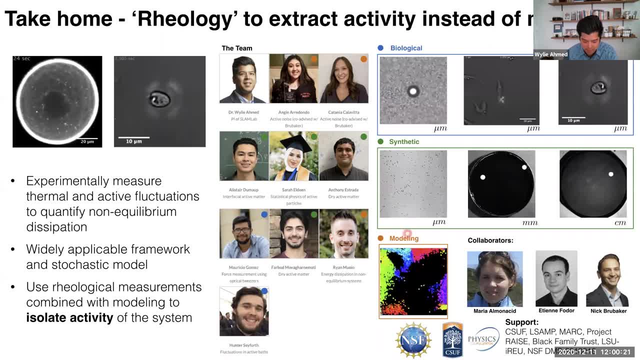 on all kinds of different things from biological systems, synthetic and also modeling, And many of them are applying for PhD programs before because, like I said- or I hope I said at the beginning, primarily undergraduate institution. So then we have many of our students here, So Hunter, Ryan, Sarah and Anthony are all applying to PhD programs. So 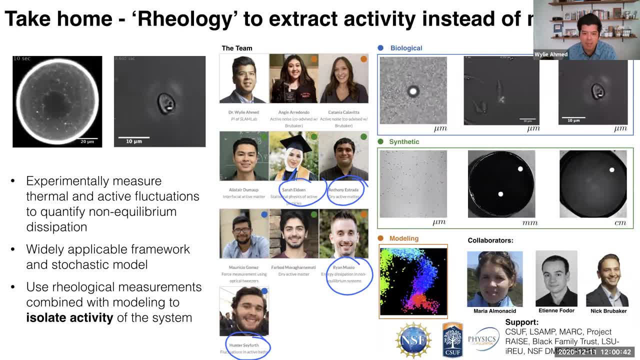 keep your eyes open. They're really fantastic students And I think I'm looking forward to what they see, what they do in their next stage. And with that, I'd be happy to take questions. Thank you, Wiley, for a great talk. So again, we will ask some questions from the chat right now. 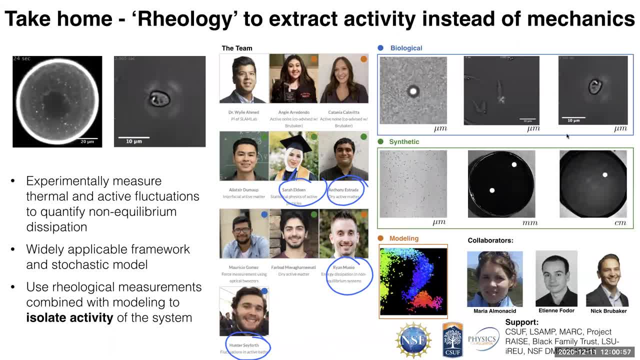 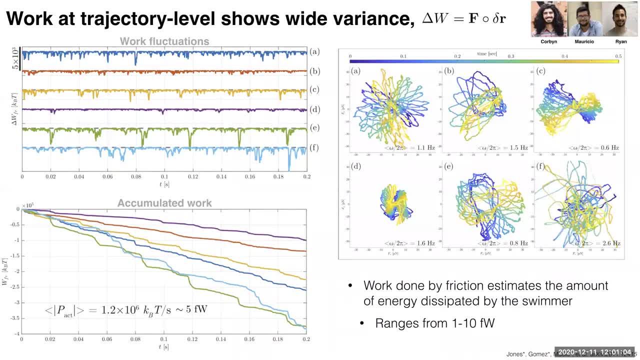 So the first. it's actually a question that's been asked a lot in the chat, which is: what is the effect of the Brazil nut effect? So this is from the slide before your fluctuation dissipation theorem slide. So this was with the cytoplasmic skeleton, if you can go back to that. 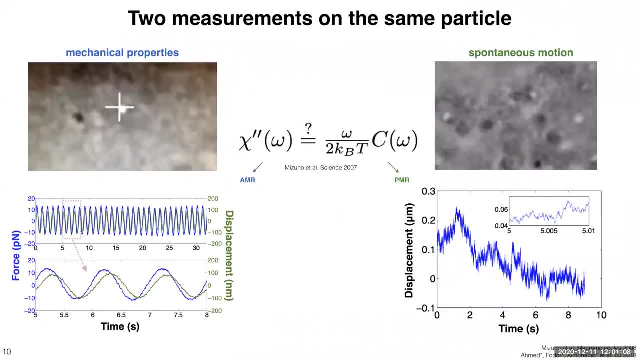 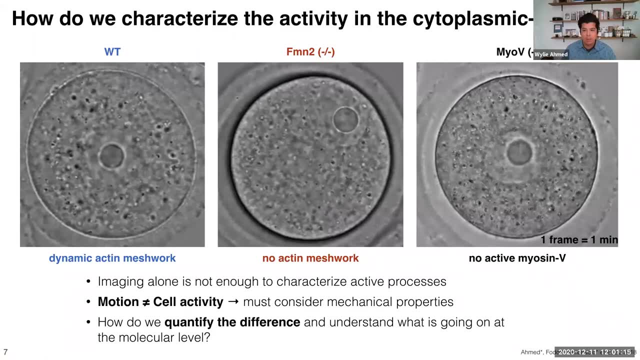 So Sharon Lopkin has a comment that this, what you described there, sounds like the Brazil nut effect. before the slide, Before this one, This one, this slide. Okay, So I don't know if you wanted to comment on her comment. 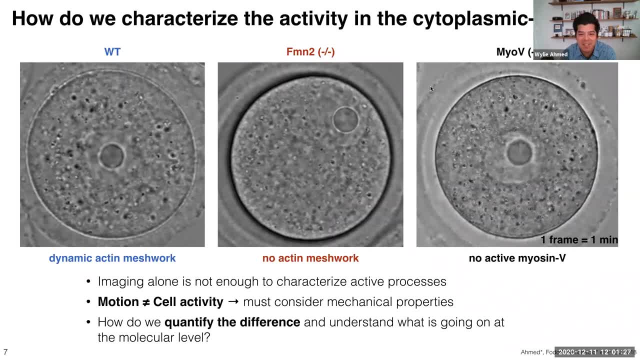 So I don't think, I don't think I know what the Brazil nut effect is, So maybe we can get to this in the discussion then. Let's move on to the next question then. And this was from Ricard Alert, And he had a comment on active fluctuation. So why are 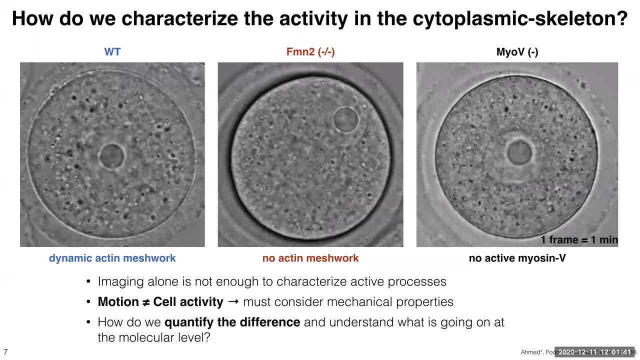 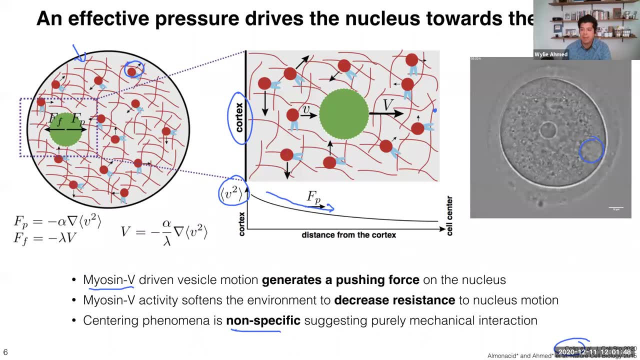 fluctuations stronger close to the cell edge? Is it because there are more motors in the cortex than in the rest of the cytoplasm? Yeah, that's a great question And don't really know the answer to that, But it seems like there's also stuff that's happening at the 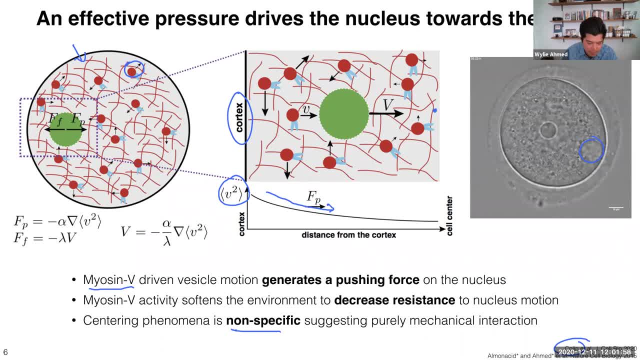 cortex actually So like in. so here I'm only drawing the stuff that's in the middle, but there's also stuff at the cortex, Like there's all kinds of actin and myosin, two motors, I believe, that are in the cortex here. So I don't. so I don't have a good question or a good answer for you. 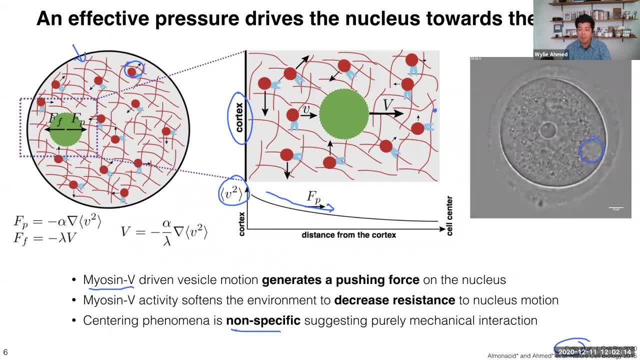 there. This is simply what we measured, So we can't really figure out why It could be due to diffusible things or diffusible stuff coming from the cortex, But it's. it's hard to say. All I can say is that 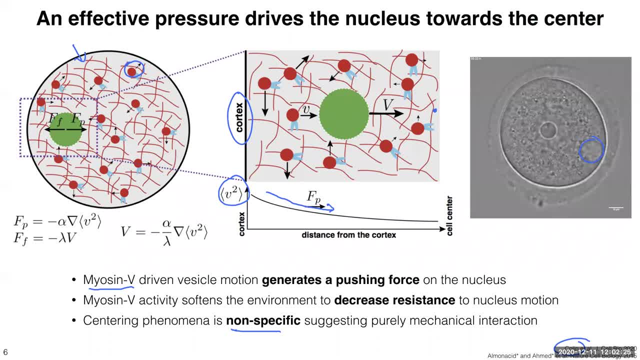 we measured it and we think it's better. Mm-hmm, think it's there. So actually, Arvind Chandrasekaran had rejoined her to Ricard's question, which was: the stronger fluctuation at the end can also be due to radial acting gradient in the system. 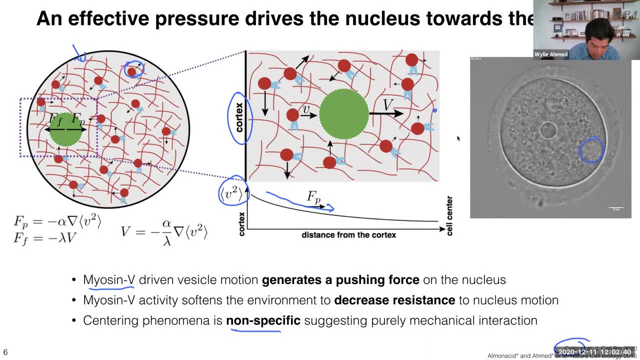 Yeah, so that's a good point And there is a gradient, kind of like there's a zone here or so where there's some gradient there, But then within side, which is still a big part of this area, here, there is no gradient that we can identify anyways. 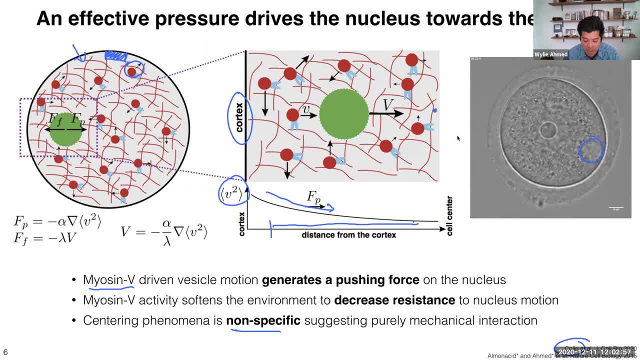 That's definitely one of the first things we looked for, And we also measured the mechanics in terms of radius. So we measured it in concentric circles going out And it was really hard to tell any difference. I mean, within our area, we couldn't tell any difference. 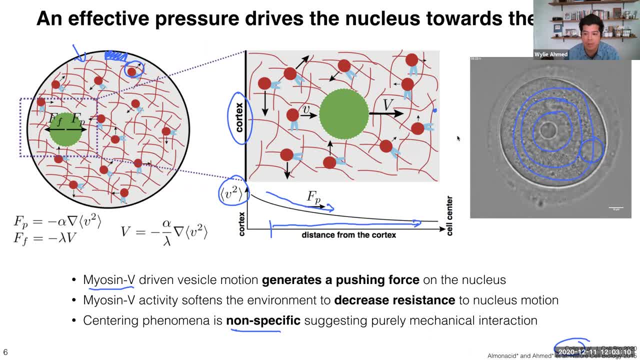 in mechanics. So it seems like it was all in the activity, Thank you. And then there's a question from Chaitanya, And their question is: did you look at the effect of active stress on nucleation? And that's a great question. 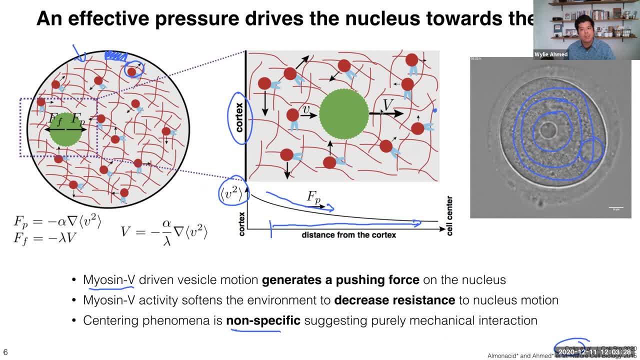 And no, we didn't In this system. we did not because essentially it was hard for us to control anything in the oocytes. So in the oocytes- that was one of the problems with kind of teasing this problem apart is anything you would do- would end up kind of killing them. 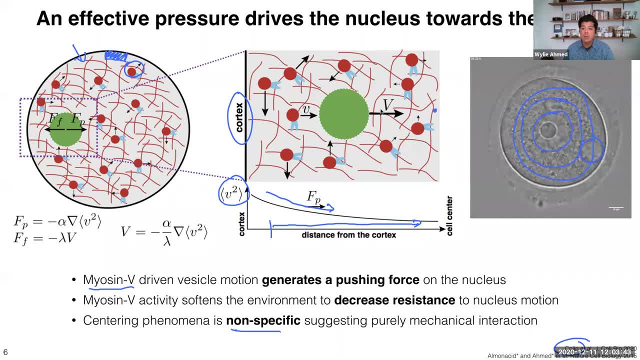 So the only manipulations we could do were to completely remove the filamentous actin or completely remove the myosin motors. It was really hard to control the degree, but that was definitely something that we wanted to do And that's something that the developmental biologists 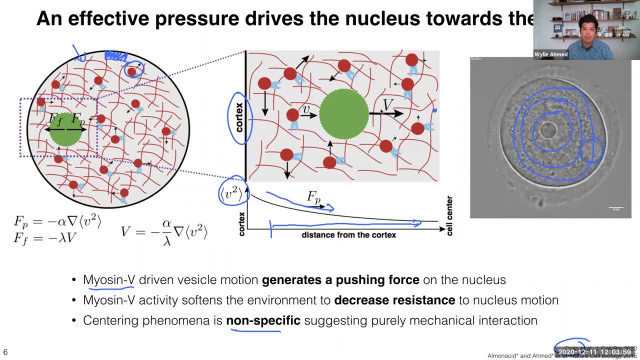 I think are working hard on. OK, All right, Then there is a question from Dave Shankar Banerjee and Robin's comment on that question. So Dave Shankar's question is: if we wait for PMR after the AMR experiment, do we expect the results? 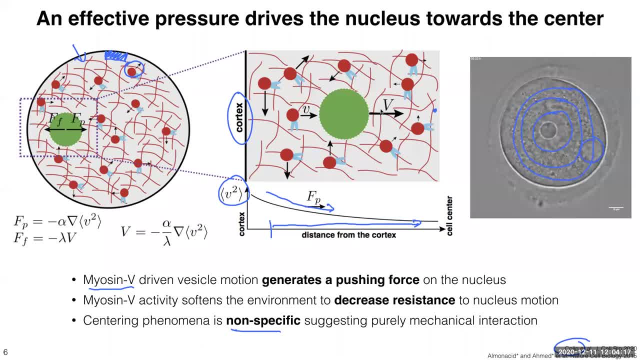 to change with waiting time? Good question, I think it depends on how long you wait. OK, So what we do is we measure them immediately after each other And we also flip their order to make sure that our active forcing is not hurting the system in any way. 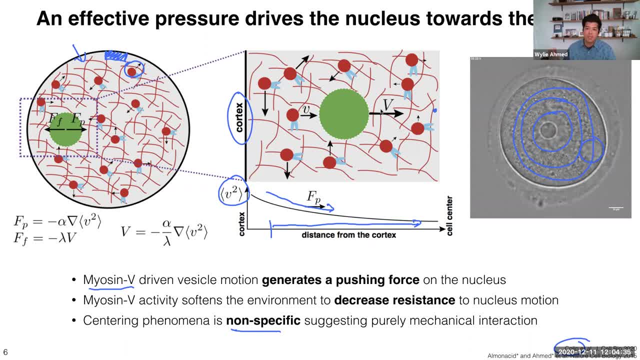 But if you, for instance, if you just measured PMR or the spontaneous fluctuations function of time, depending on your system, they will change In the oocytes. they will only change if the kind of the stage of the development changes. So they're very stable, which is why